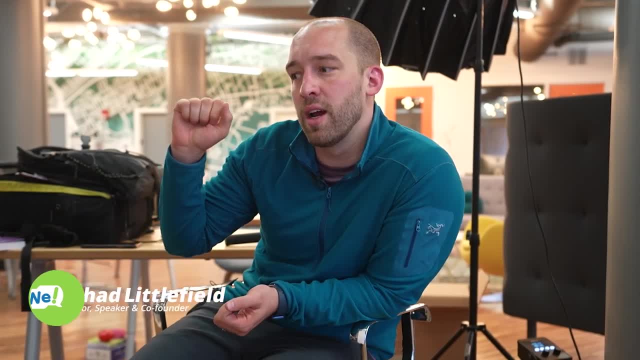 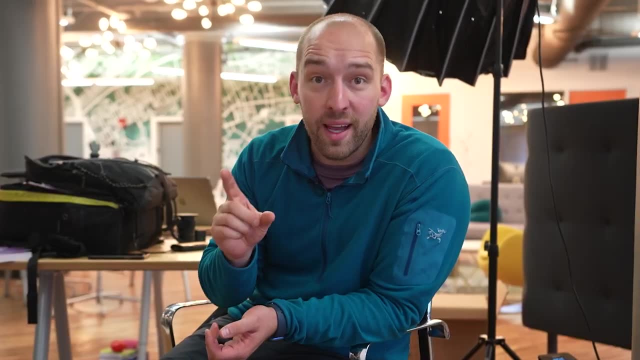 I get to do this for a living and so in this video I'm actually going to share. these 10 exercises are signature exercises that I use with some of the smartest leaders and educators on the planet that I work with. If you pick even one of these to do with your group or your team in the next week, 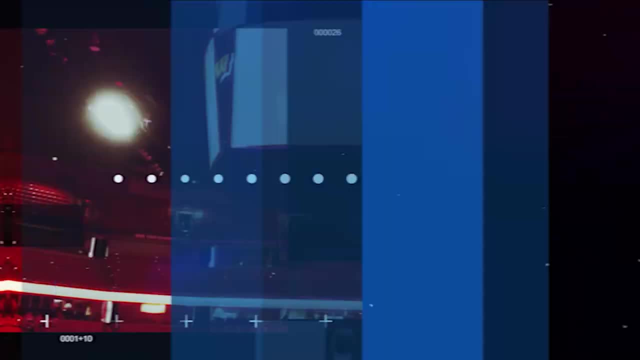 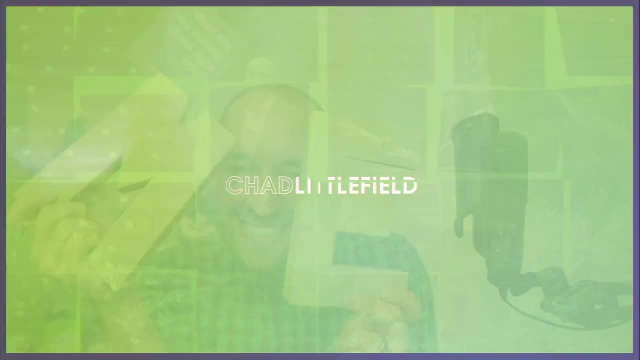 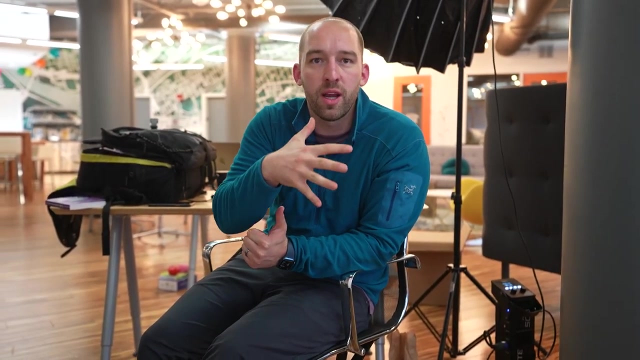 you will see engagement go up, and if you don't, you can write me an angry email. 10 is a lot, so to segment our brain, I've actually divided them out. I have discovered over the last several years, working with some really cool organizations, that there are five ingredients. 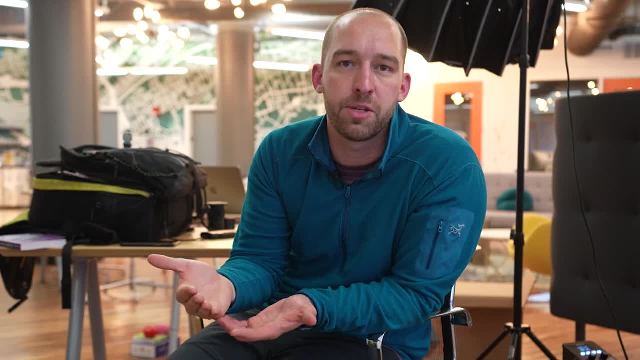 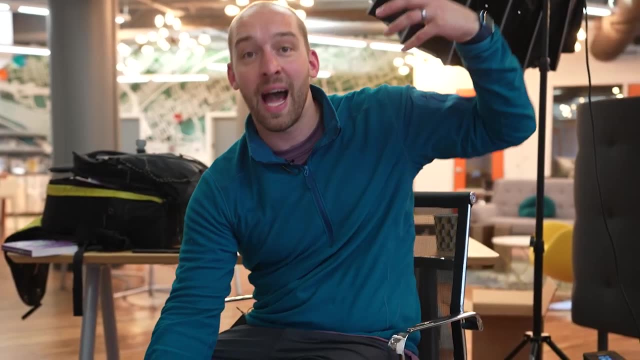 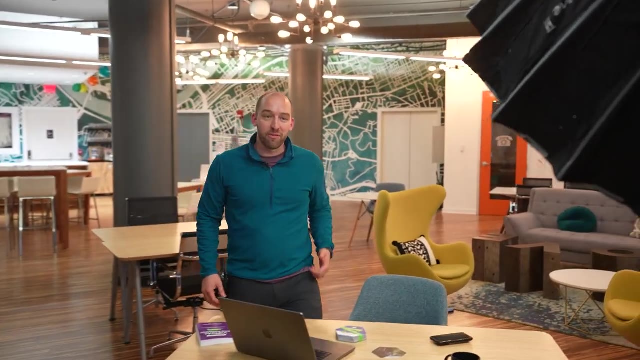 that consistently increase engagement, And so I'm going to share two exercises at each ingredient that you can make come alive. and the first one- the reason I'm starting behind the scenes of filming- is this concept of an unofficial start, And so the idea of an unofficial start, which I learned from a lovely fellow in Australia named 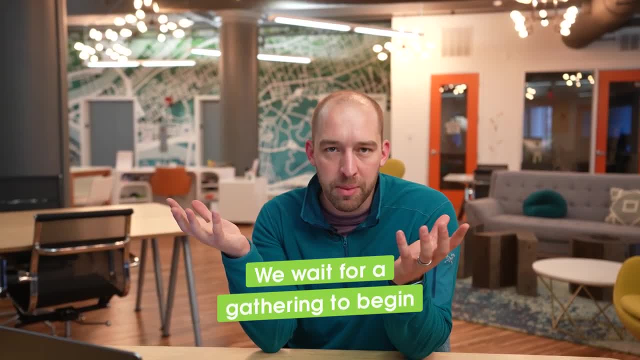 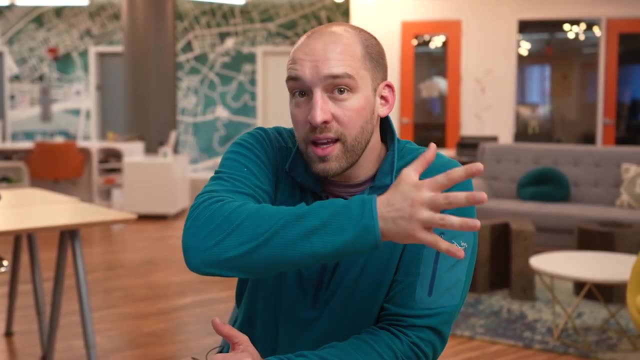 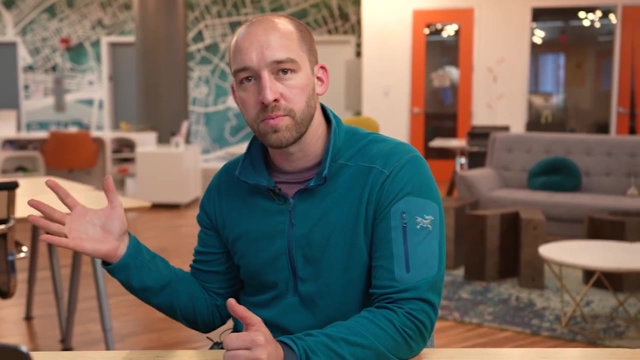 Mark Collar is the concept that typically we wait for a gathering to begin, as opposed to starting immediately with purpose, And so unofficial start is something that can happen before the actual official start time of your meeting To spark engagement in the first minutes as opposed to waiting. 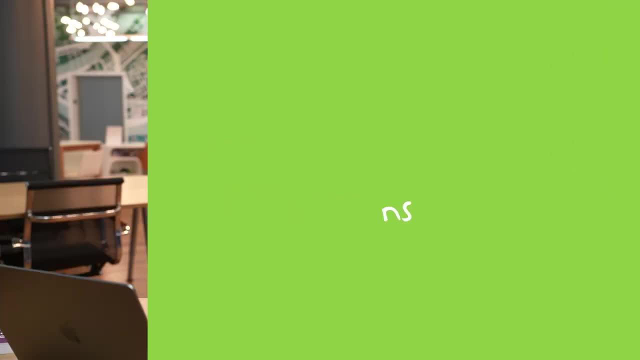 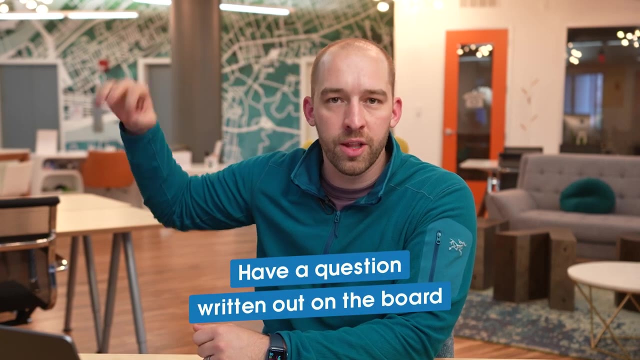 The first activity I call anchor questions and this is like on a whiteboard as people come into the room, or a chalkboard or a flip chart piece of paper. Have a question written on the board that you want to refer back to people's answers throughout your meeting or gathering. 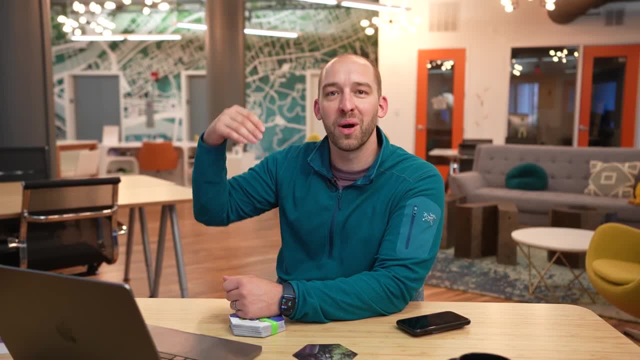 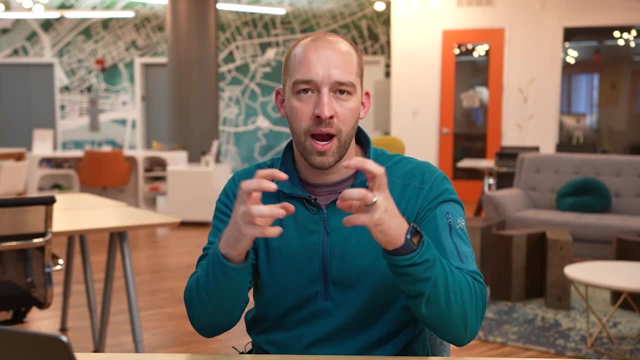 Right. so the question might be: what is one thing you want to get out of today, or what is something taking up lots of your brain space right now? What is the challenge you are up against? Right, some anchoring ground. This is a very grounding question that you can actually tie your content and the rest of the meeting to throughout. 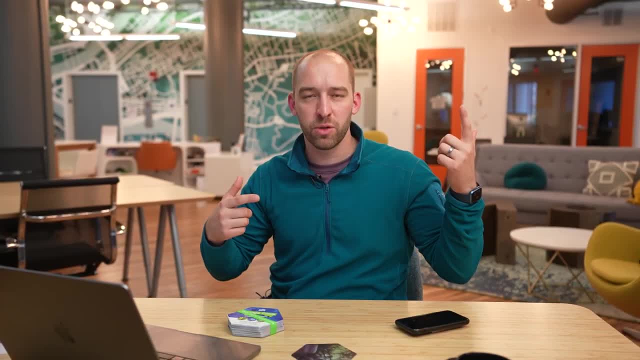 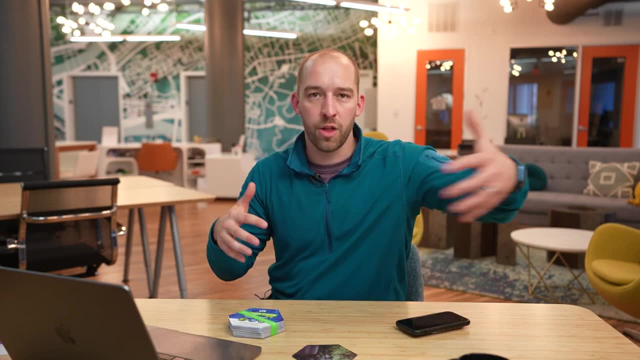 One bigger one that I like that might take some thought for people to respond to is: what is one thing you're intending to achieve at work Right, because ideally the purpose of my meeting or gathering helps other people accomplish their purpose. So when I know what they're trying to, 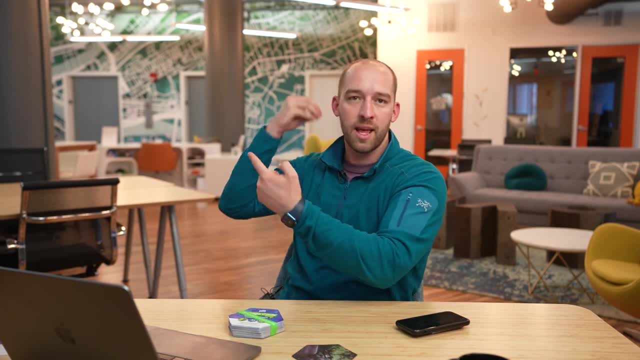 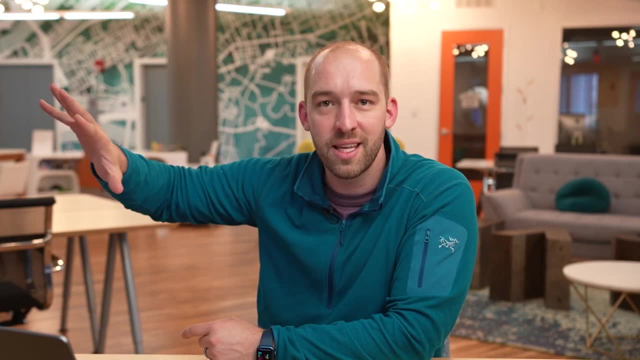 achieve. I can anchor everything else that happens in that meeting back to it And so really simply writing that down and inviting people to write their answers so they're visually displayed- Everybody can see them. You or anyone else can see them, Anybody else can, and when you do this, they will point back to responses to be like: wait, we got off track. 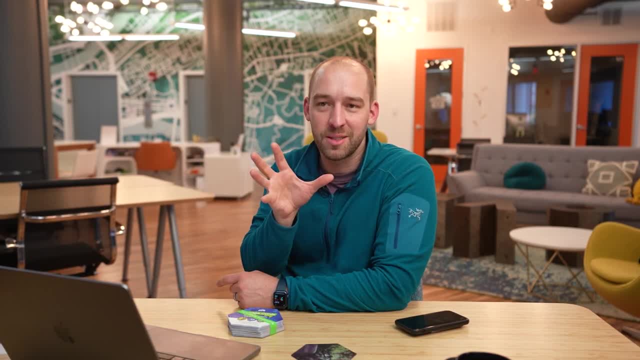 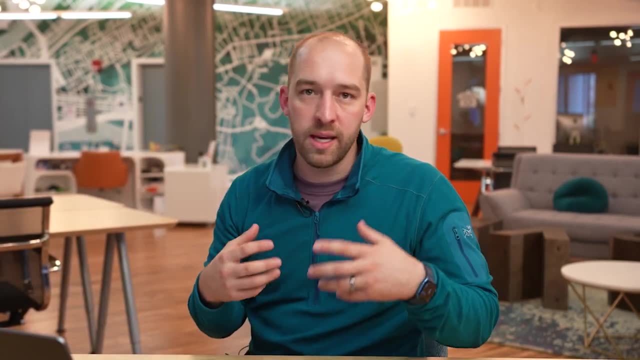 Remember this is why we're here, right Anchor questions. Second one, and remember, unofficial start ideally is something rolling as people are coming in, You don't? it does not require everybody to be at the gathering, workshop, training, meeting, off-site. 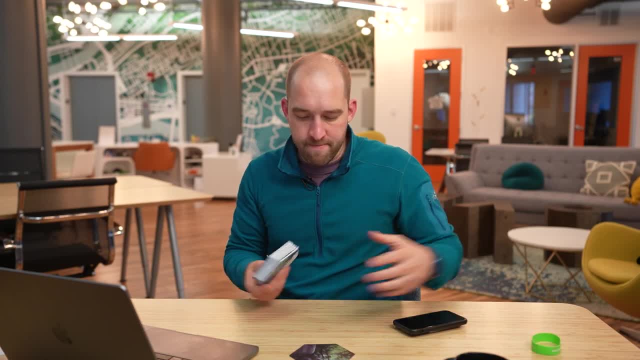 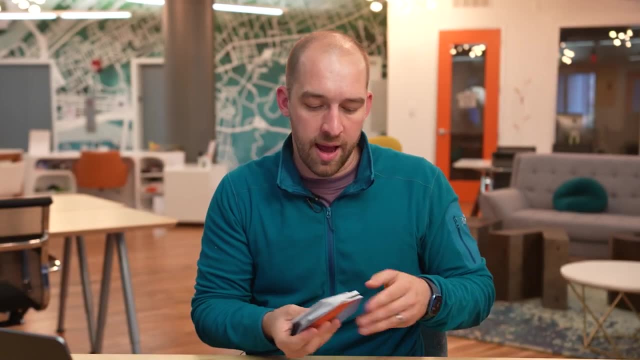 conference, whatever it is, And so this one just uses quotes really quickly So you can print out quotes. I happen to have a deck of cards called we engage cards that have some really lovely quotes and images on the back, And so I just spread them out all over a. 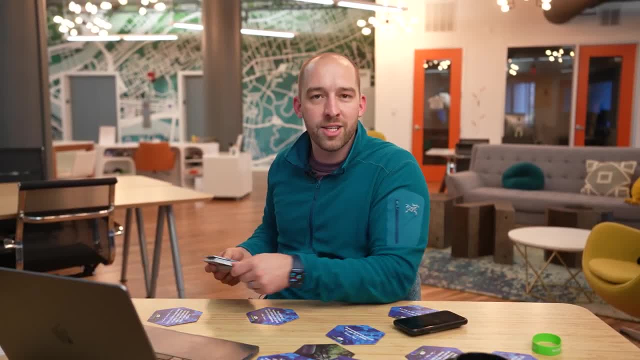 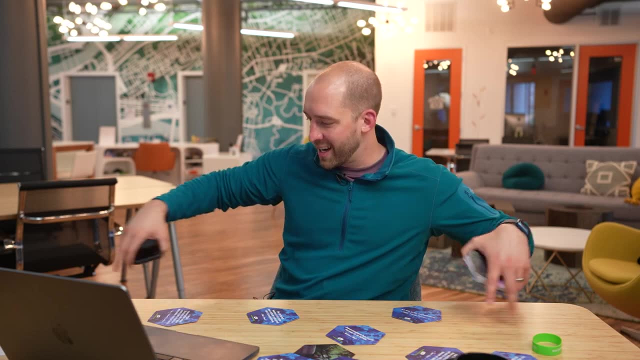 table and as people walk in. I just did this in Wichita, Kansas, not long ago with a group of lovely faculty And as they were walking into the room, I just said: can you choose? I moved my phone off the table and I just said: can you choose a quote that you're clicking with right now? So I 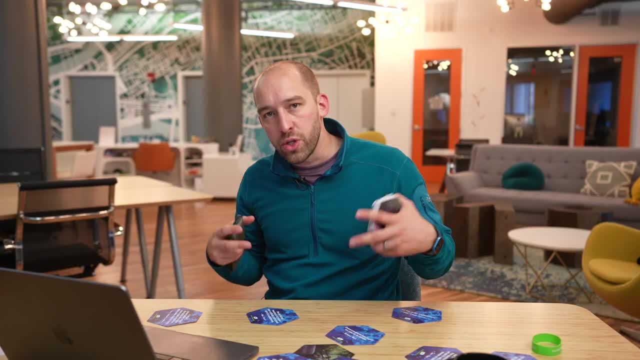 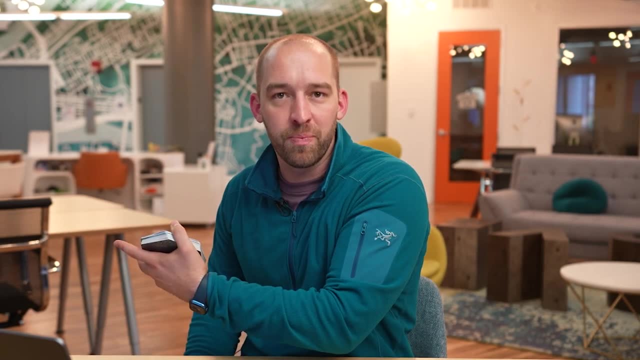 call this click quotes. So, as people are walking in, can you choose a quote that you click with right now and just sit down next to somebody and share your quote? And I'm going to go ahead and share my quote and why it clicked with you. Really simple prompt. I say it individually, I don't 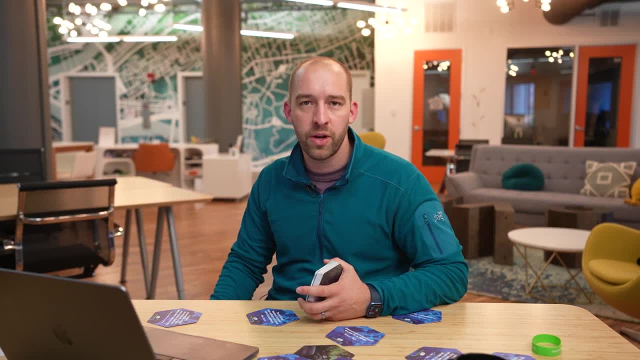 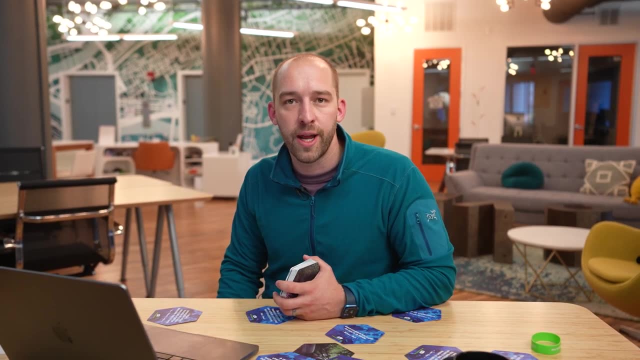 announce it. It's not a big like we're doing this, It's like: hey, welcome, super glad you're here. As everybody else rolls in, can you just choose a quote that you click with and sit down and share it with the person that you sit down next to as you connect? This is a really good point for me. 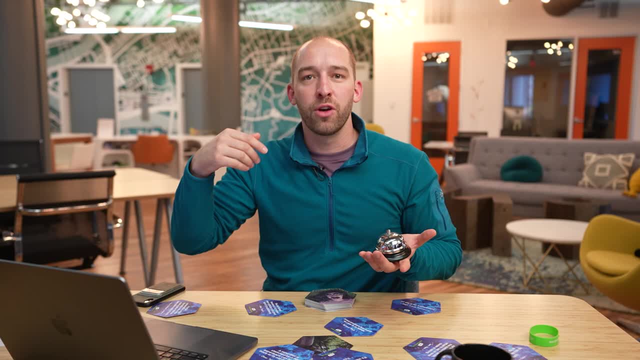 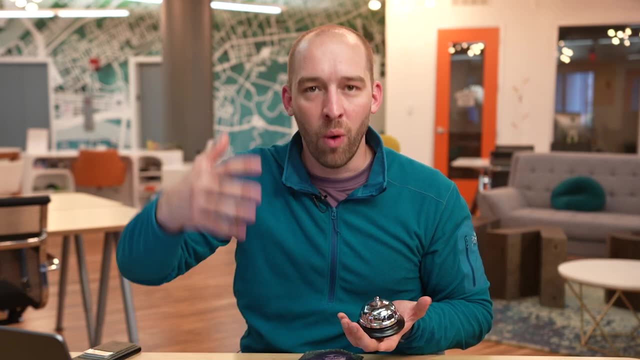 to remind you, as we go through the other exercises in rapid form, for you to ruthlessly steal and reinterpret any of these ideas to your own context right. I'm not facilitating this activity for your own sake. I'm just going to personalize my framing around it and make sure that it fit and tied and 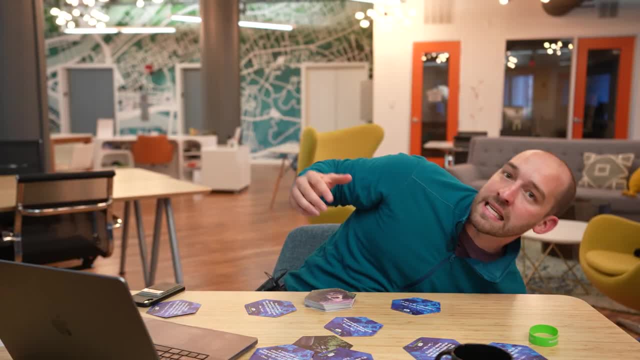 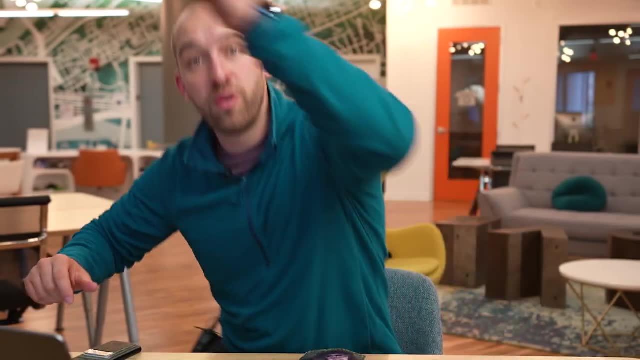 connected to the purpose of what you were doing, And so you need to listen to all of what I'm saying through the lens of how can I adapt this and make it fit my group really, really well. So, as we move into the second ingredient for engagement, think about. you know how I might. 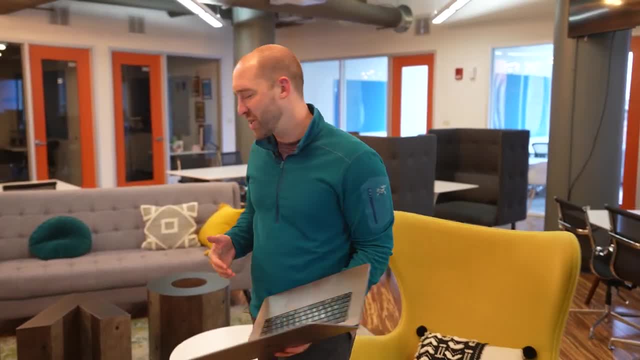 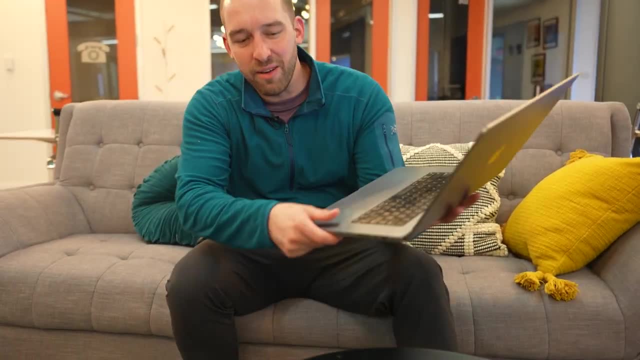 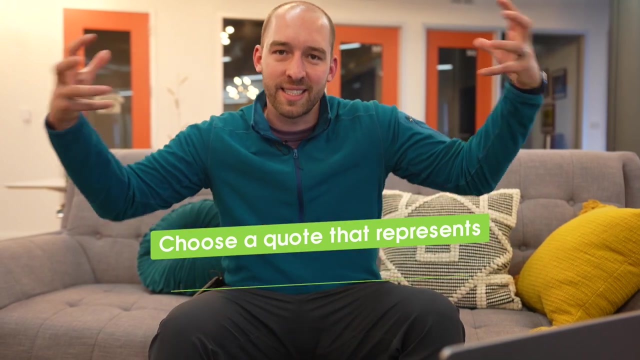 adapt that quote quick or click quote exercise. If you were meeting to come up with the mission, vision, values of your organization or your committee or whatever else, or decide the theme for the conference this year, I would say: choose a quote that represents how we. 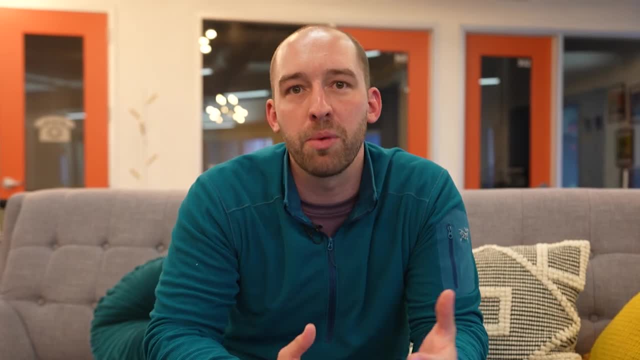 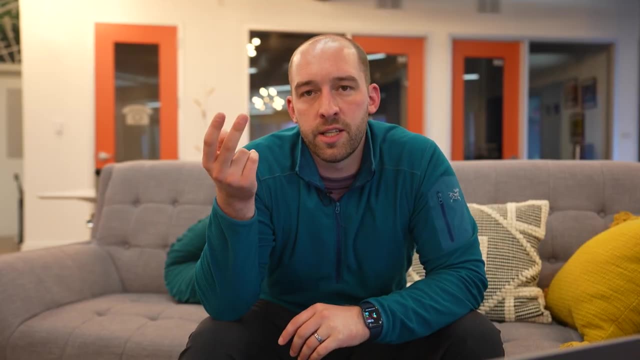 want people to feel when they leave our event, Or choose a quote that represents how people, what people will be thinking about when they use our product or service. Second ingredient is this concept of a context hook And the idea is, even if you're meeting in person or virtually, when people 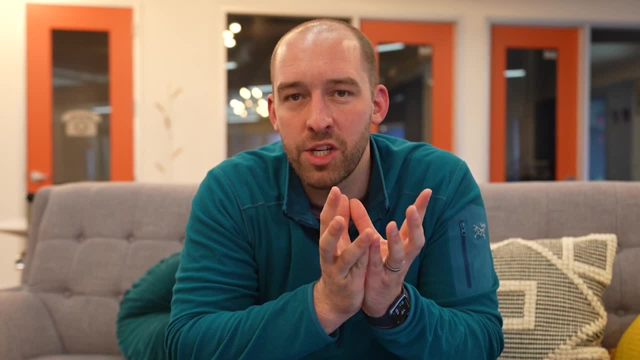 walk into the same room. I don't believe they're in the same context. They're not actually present with each other because they're living probably either in the past or in the future, And so I'm going to talk a little bit more about that. in the future of what they have to go, Most likely, whatever- 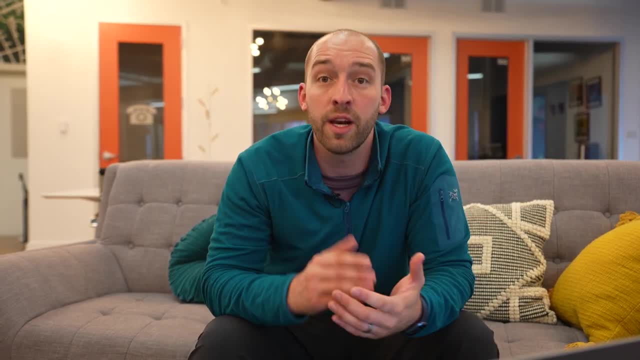 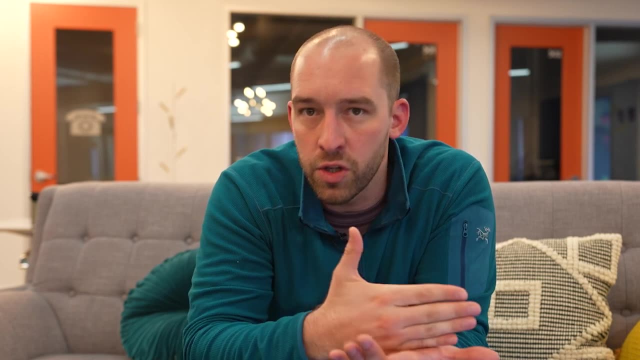 has been happening before is still in their brain as they're entering in that meeting, And so you've got to do or say something really, really quickly. So one of my absolute favorite exercises to make this come alive that I've been doing in small groups of 20 people, which is a small group for 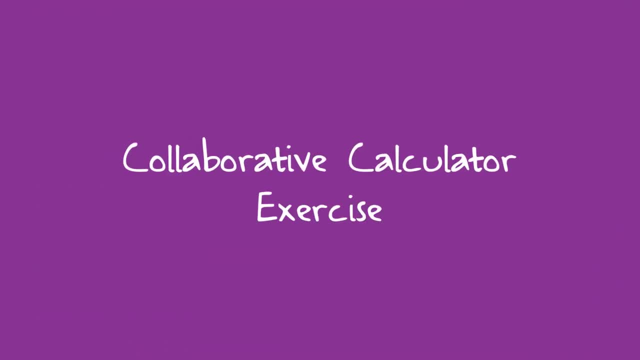 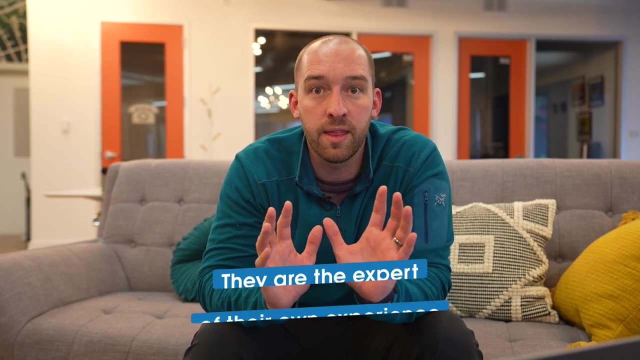 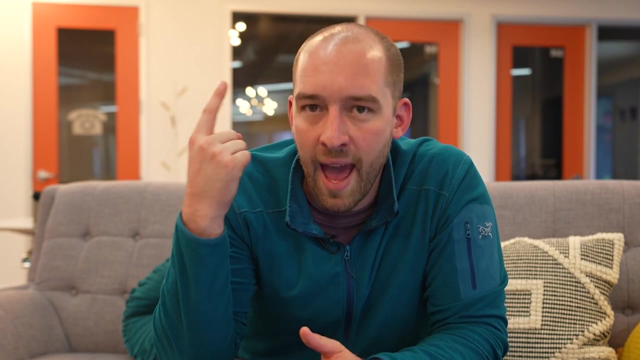 me, or a large keynote with 2,000 people, And it's the collaborative calculator exercise And really simply, it's my way of walking into a room humbly, with the perspective that they are the expert of everything, And so I ask people to come up and calculate the number of years of experience that 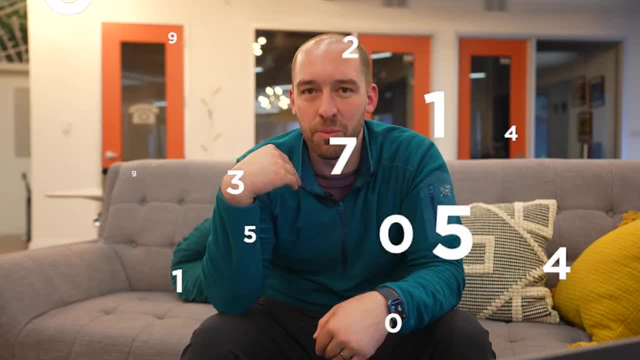 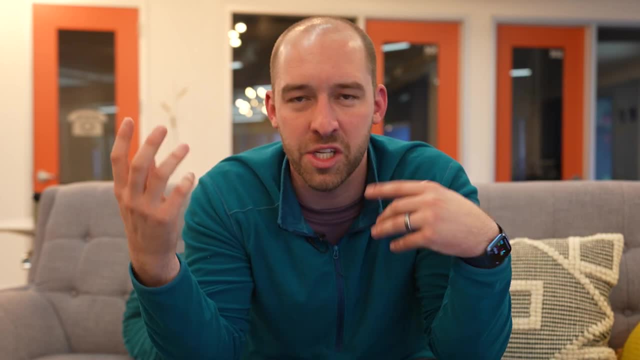 they have in their niche, And then I have them popcorn it out, Shout out a bunch of numbers to me And I listen to those numbers and I say: okay, what do you think the average of all those numbers you just heard is Just? We're just doing some collaborative calculation, Not exact math, but we're getting close, So let's say 15 years. So I was a few weeks ago speaking at a conference in Orlando with 500 internal auditors And the average years of experience was about 10, which was good for 350 to 500 people. I didn't count in the room So I said let's just On the low side- 300 people. 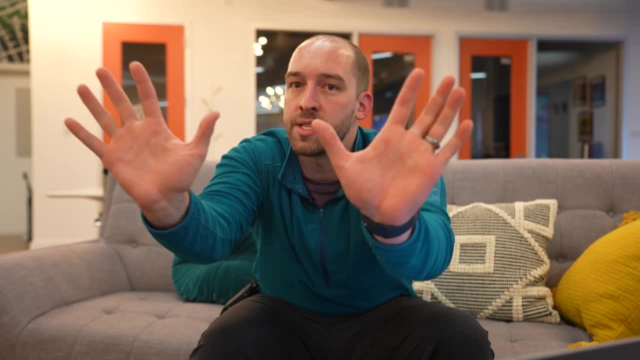 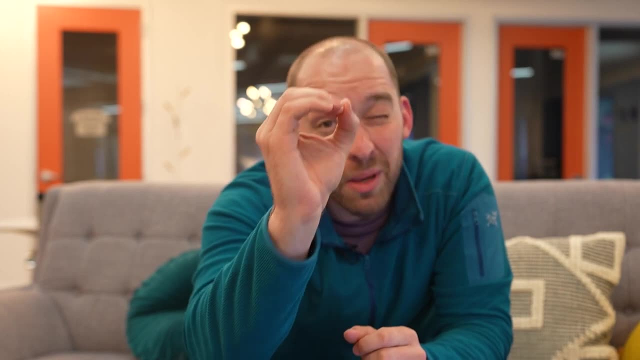 in the room average of 10 years of experience. That means that on this side of the stage, there are 3,000 years of life experience and wisdom, which is why this is the number of PowerPoint slides I'll be using today and why I've designed the session for contribution and not consumption. 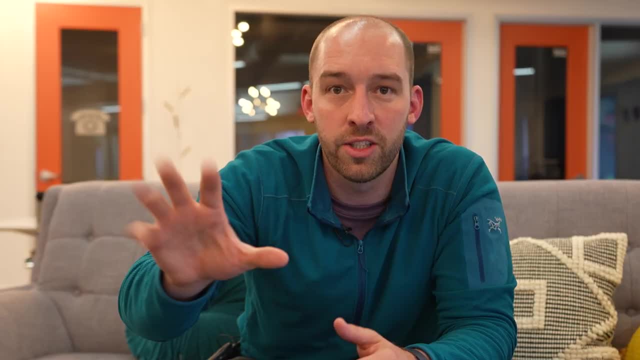 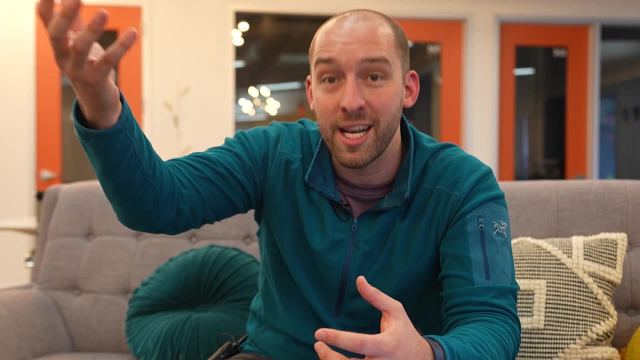 right, Because you collectively are smarter than I am individually, So you can see how that quick exercise and coming up with a number of years of experience in a group actually really brings to life like. this is why we're asking you questions. This is why this is. 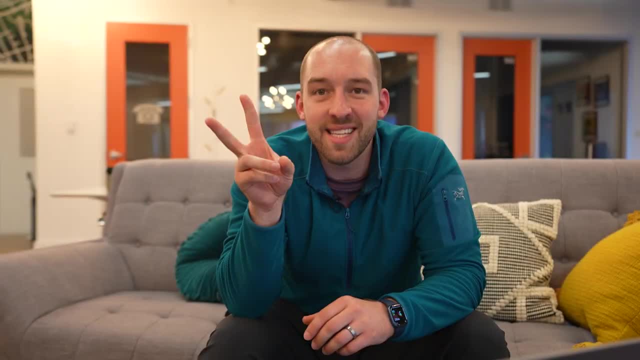 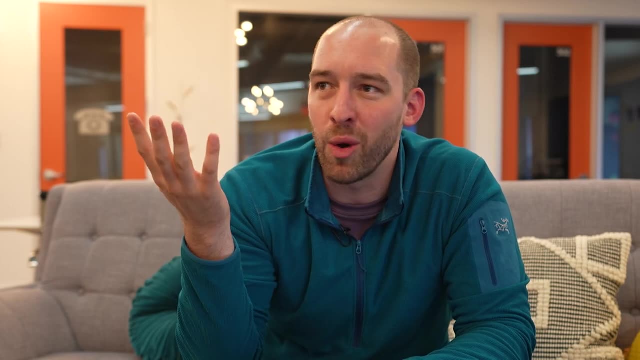 a discussion. This is why this is not a one-way meeting. The second exercise I literally did two days ago for the very first time and it was pretty cool. So, ironically, I'm in a building right now in my old office space, which is the co-working building, and I'm in the community floor and the 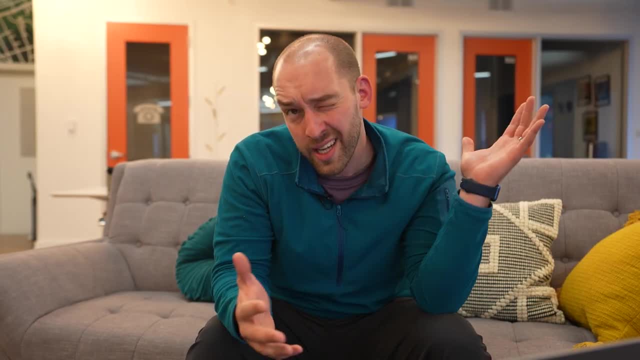 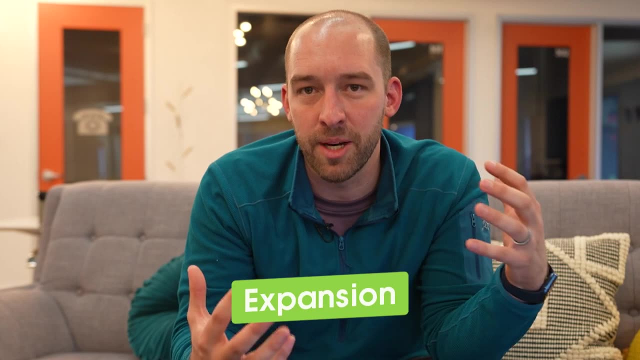 space is called expansive And, ironically enough, or coincidentally enough, I don't really know how to use those words. Two days ago I was speaking at a conference and the theme was expansion And I was trying to think of what is the context hook that I can come up with to invite expansion to. 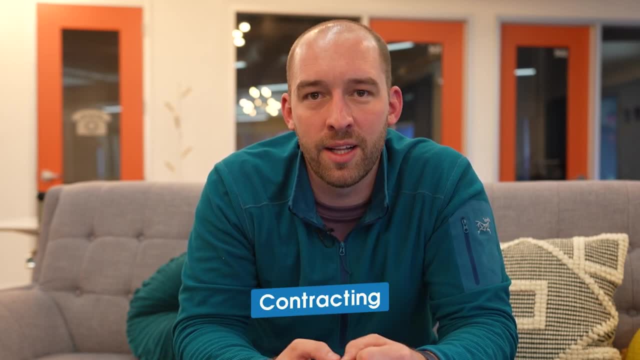 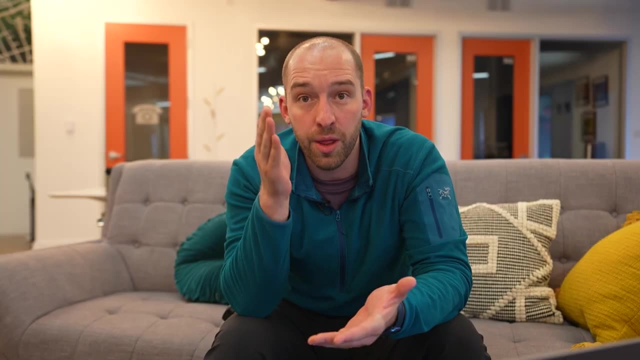 happen And I thought of the opposite of expansion, which is contracting. And so you can do this with me as you're watching this video and viscerally embody this idea, and it'll help you remember the exercise too. So I want you to think of and actually target a muscle in your body somewhere, So think. 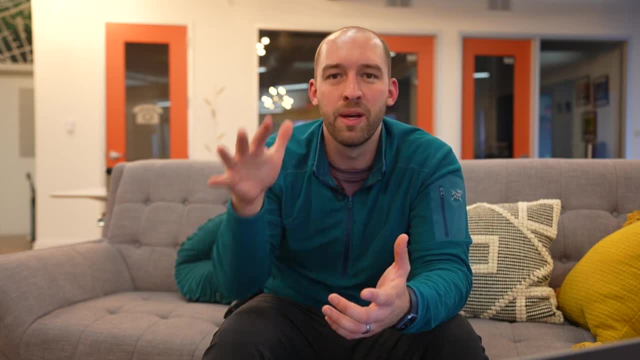 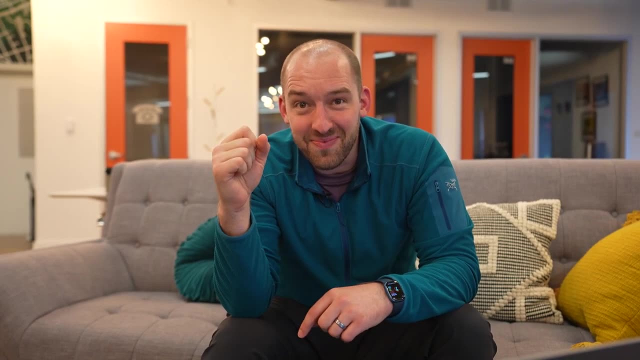 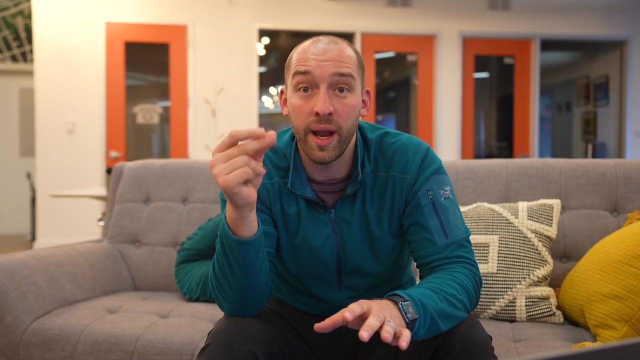 of a major muscle group, So like a bicep, a quadricep, a glute, Think of a major muscle in your body and contract it And release it. So now round two, Ideally. context hooks, by the way, are quick, I told you. 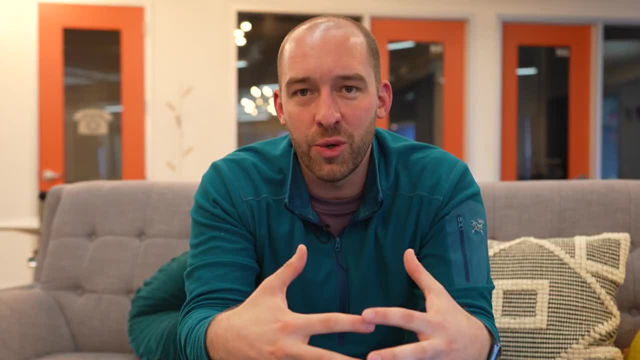 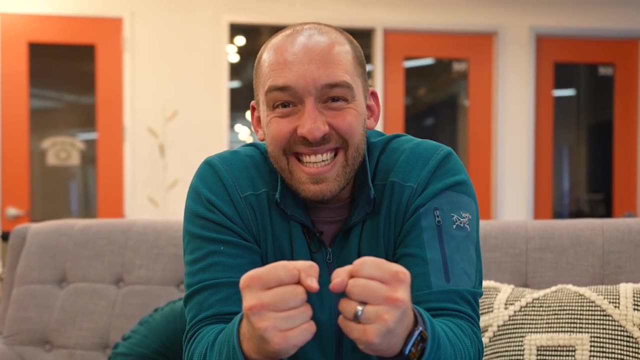 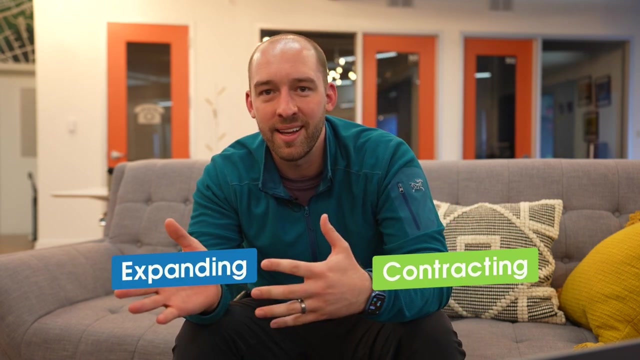 these are quick exercises. Second one: now take every single muscle in your body. Don't pee yourself, but flex or contract every single muscle And expand. And then I just simply ask the group which was easier, contracting or expanding? I think sometimes we approach expansion within a state. 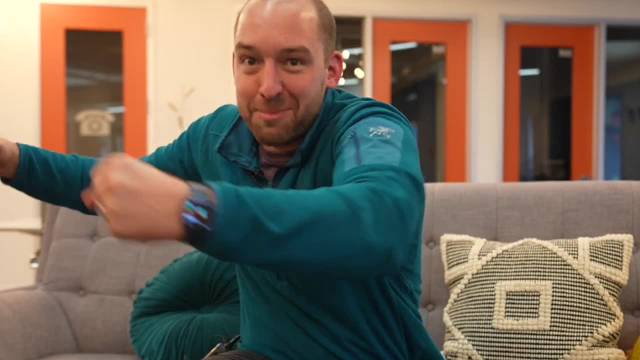 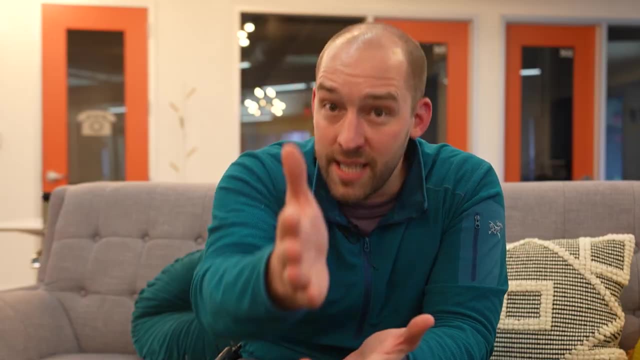 of contracting where we're like this, We're like need to do work, Work to expand, expand, expand and grow. But what if we actually approached expansion with a different layer of lightness and allowed us to expand right, So you can take that exact exercise and use it? 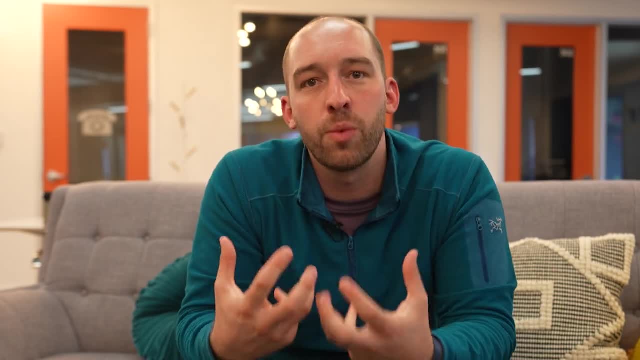 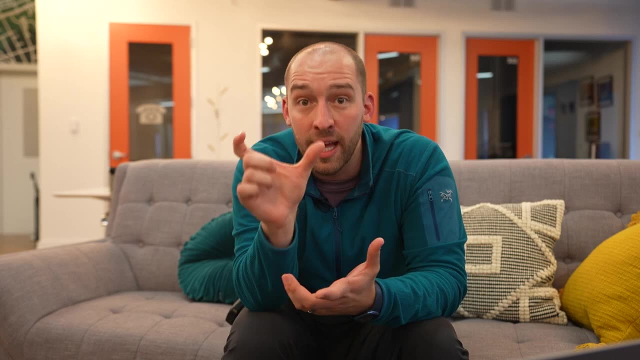 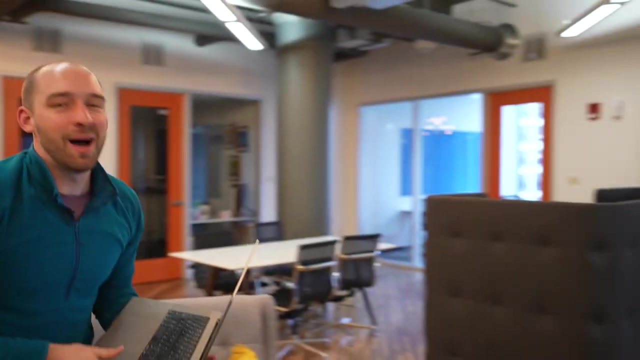 and apply it. But the idea is that I did have them do something that connected with their body, that put an ethereal concept into a concrete experience. that took less than 60 seconds. I like context hooks that take less than a minute. Next two exercises: so delicious. We need to shift gears. 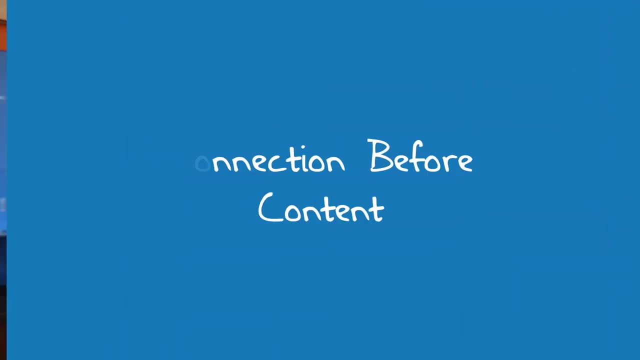 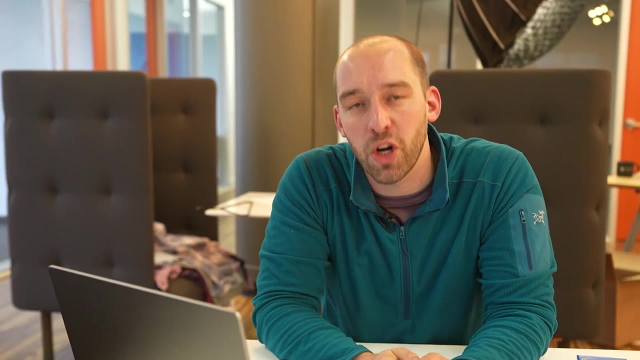 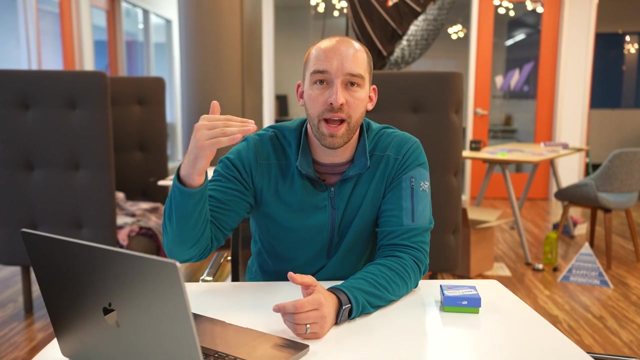 for this one, though. So connection before content, Oh my goodness. If you want to increase engagement in your group, stop doing icebreakers, Stop doing icebreakers and start doing connection before content. And the difference is: connection before content must connect to the purpose of why you're actually there. 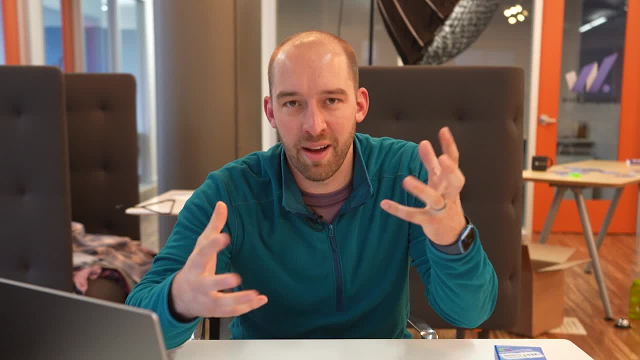 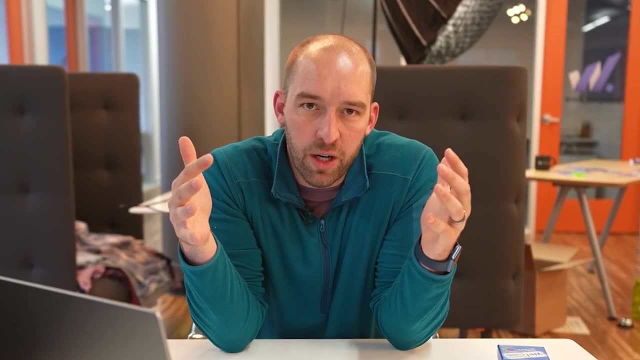 in that gathering or meeting or conference or summit, etc. One of my absolute favorite exercise I call teacher mode, which is why we're at this like teachery little table here and I'm in teacher mode When you say icebreaker to a group of software engineers. 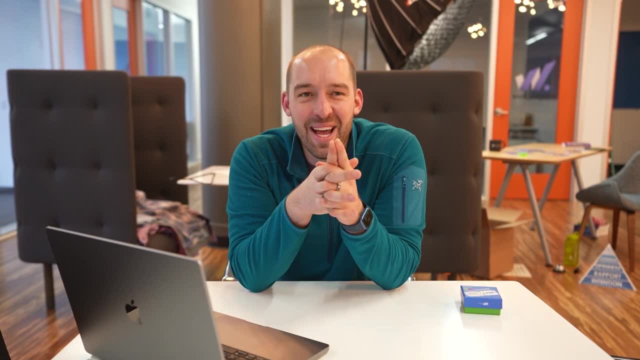 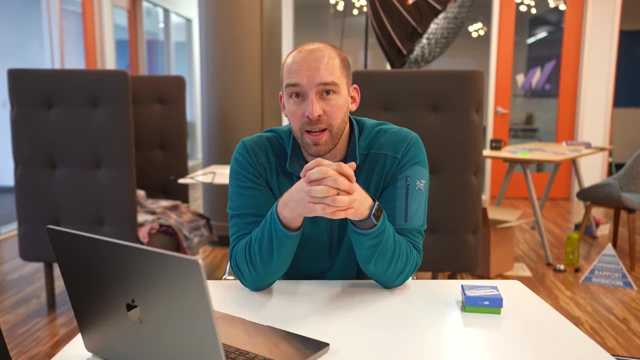 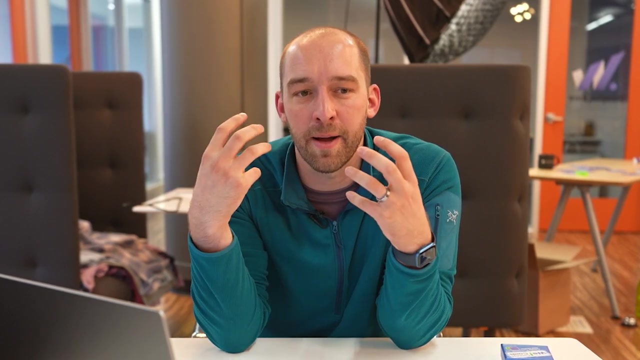 eye roll right When you say icebreaker or let's do a little warm-up activity to a group of just about anybody. actually, there's going to be a percentage of that group that gets hives- Either mental hives or physical hives- when they hear that idea. And I think the reason they do is because 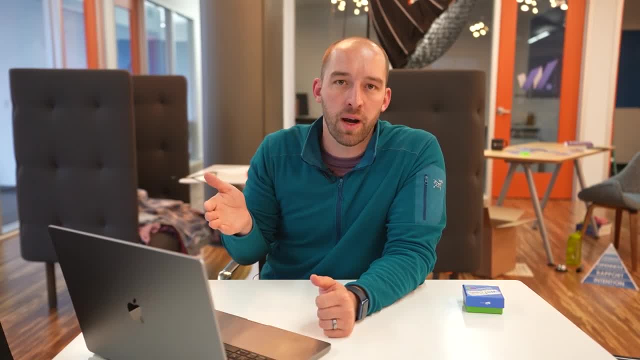 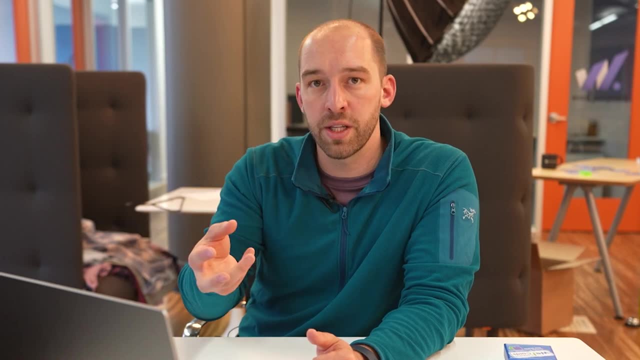 it's not connected to purpose, And so, ideally, when I do connection before content, I'm thinking about how can I make this super, super valuable for the person. So if they actually engage in this, they will leave the conversation smarter, wiser, They might have an idea to save them time. 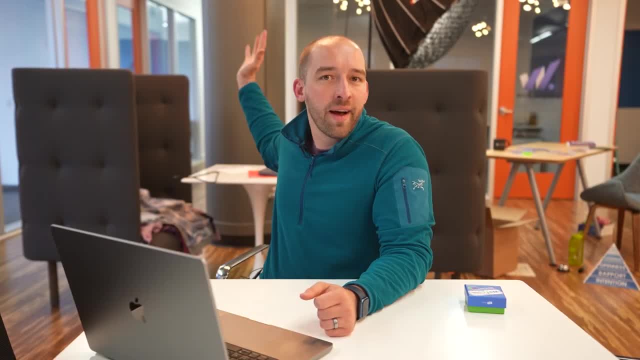 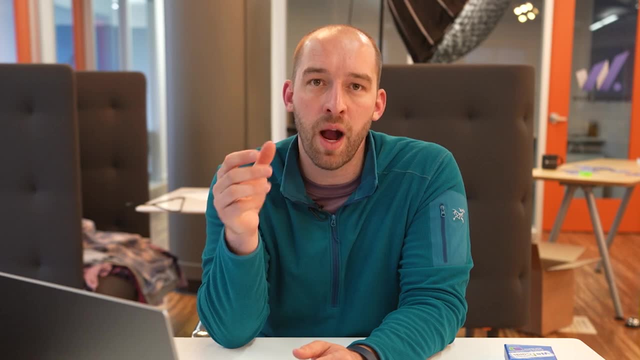 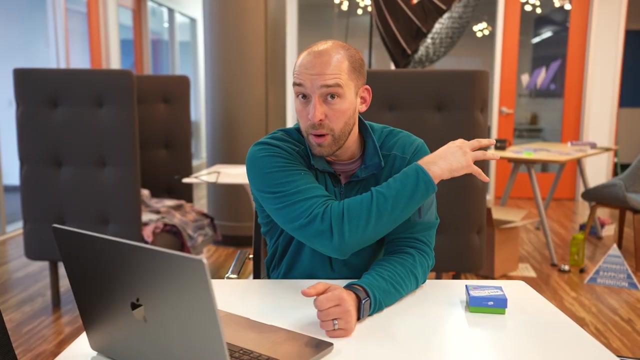 etc. Not, they're going to learn the favorite color of a colleague, right? Nothing wrong with that. But in teacher mode it's a framing idea where I come up with a question that I think, if answered in a small group, will create a goldmine of wisdom. right, It'll access that collaborative calculator. 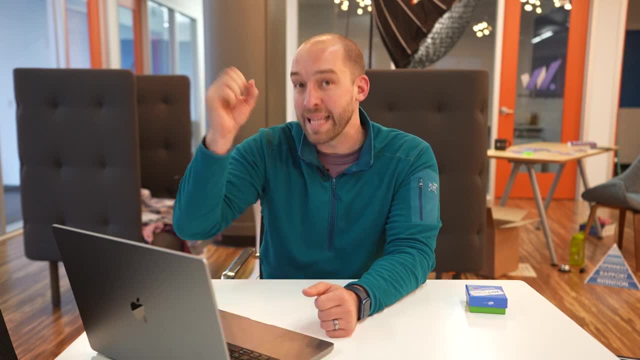 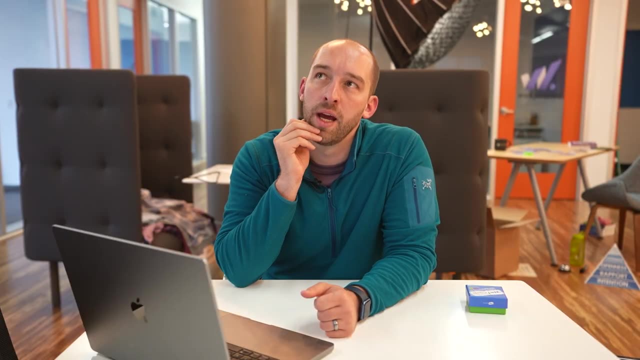 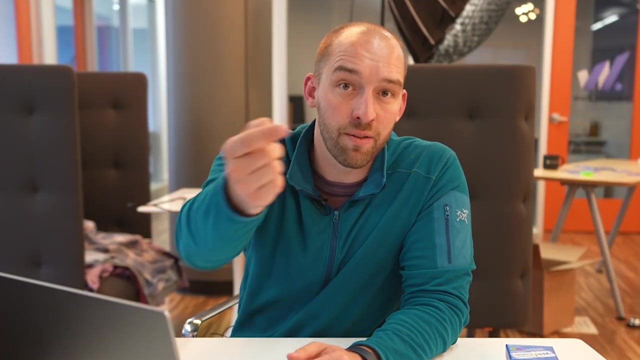 exercise I shared earlier. It'll draw out some of those millennia of experience, or some of those ideas out and share with the group, And so it might be a question like: what is one thing that saved you time in the last 3 months? Because, if I know the answer of 3 other people to that question, 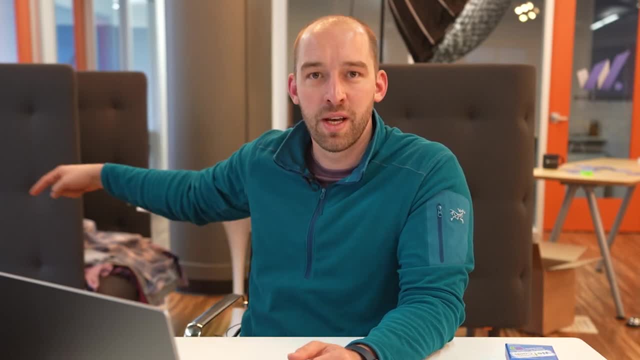 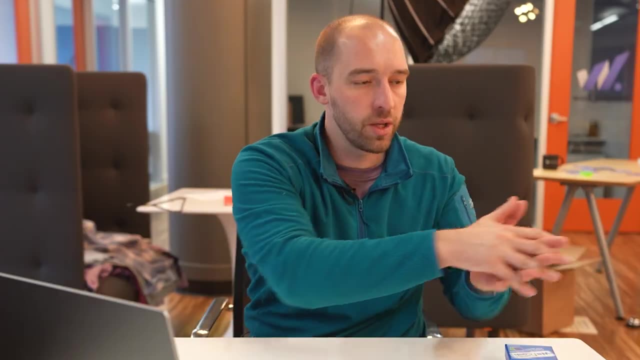 it's possible that I'm going to save time in the next 3 months. So this teacher mode is really simply inviting people to be a teacher of something useful as they answer the question that is posed. So really simple. It's a connection before content. question: Getting people ideally into troubles, or 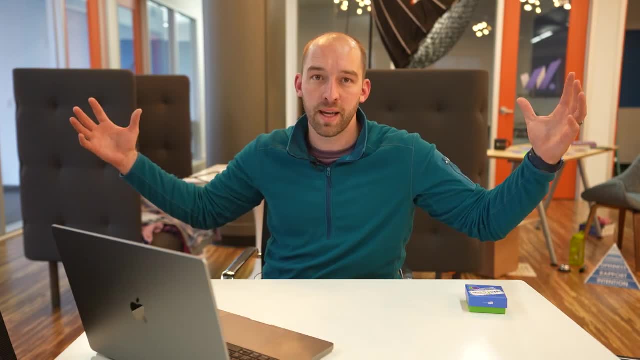 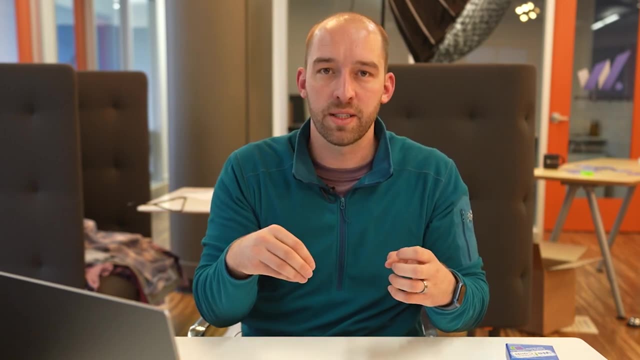 quadruples, Not bigger than that. I think bigger than that is public speaking, And so you like to keep it small. 3 to 4 people Get in the conversation about a question that will add value to everybody else. that allows you people to connect with each other. connect to the. 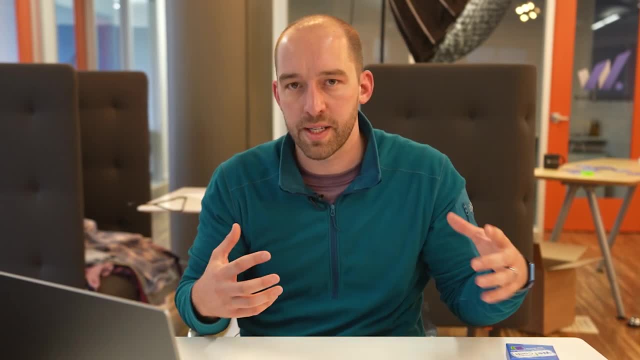 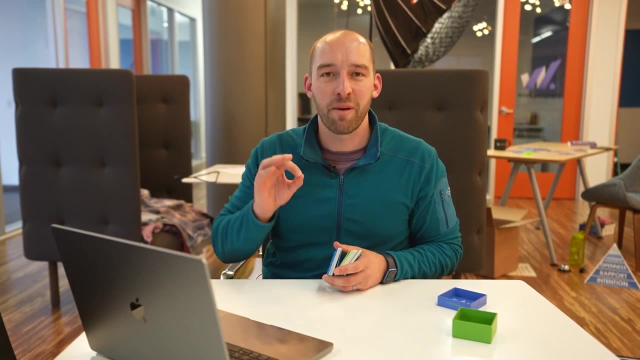 purpose of why they're there and ideally, gives people the option or choice for authenticity and vulnerability. Second exercise: This is one that I've shared, but I cannot help share it again, because it is absolutely one of my favorites and it's never failed right. So if it fails for you, 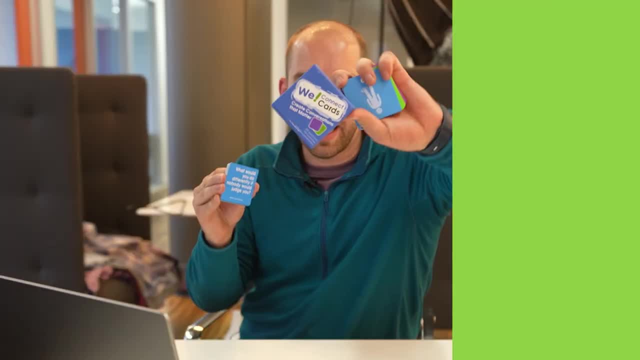 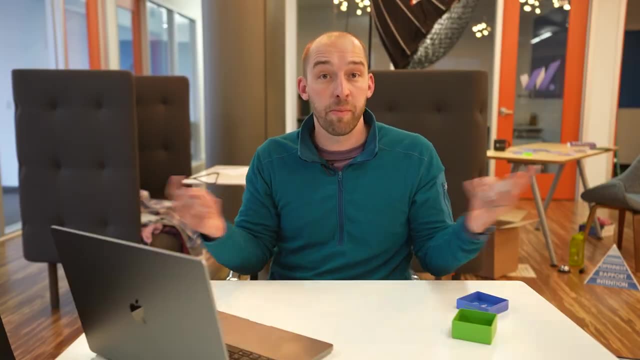 you need to email me and tell me why Question swap. You can use WeConnect cards, which is a deck created that's linked below and it's being used in organizations and schools all over the planet to help make connection really easy and create conversations that matter Really, simply, though. 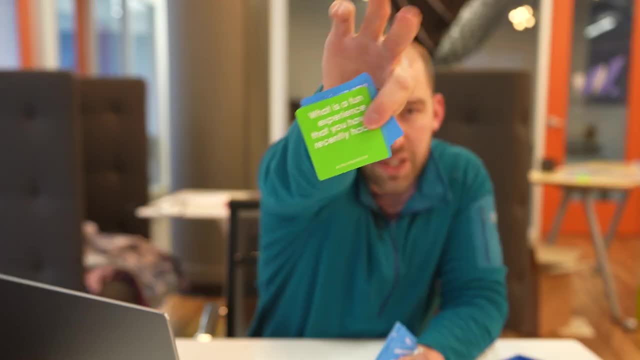 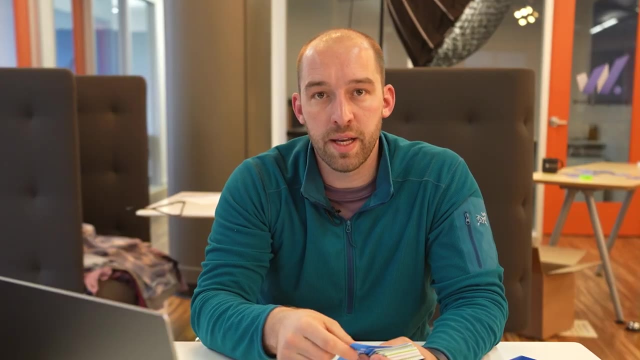 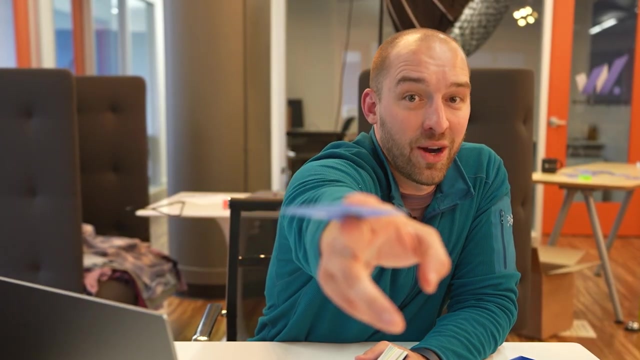 there's a question on each card, and they're questions you normally wouldn't get asked, Right, The mechanics of this are: what is the golden part here? The question swap is: everybody gets a card. So Steven hand, You get a card, and other person in the group, you get a card. 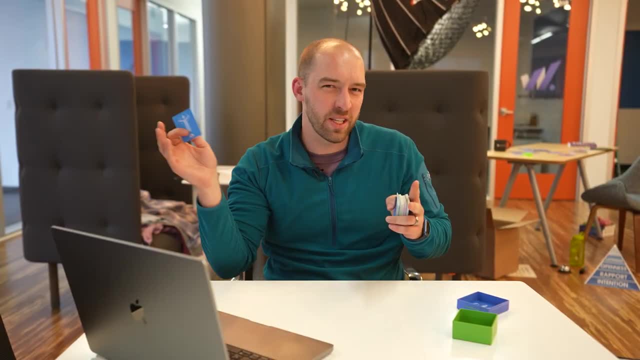 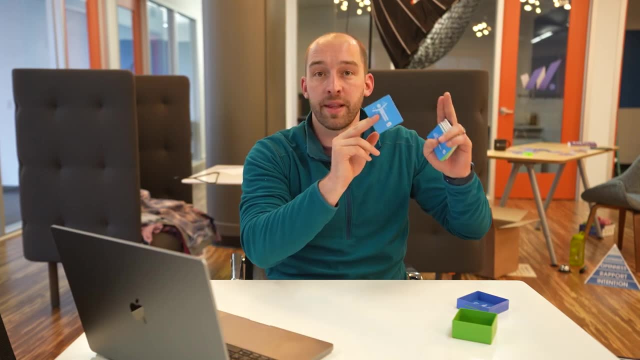 and I get a card, And this works for groups larger than 12.. It does not work for smaller groups than that. You can make some adaptations, but I invite people to stand up and pair up with the person that they know least in the room, So 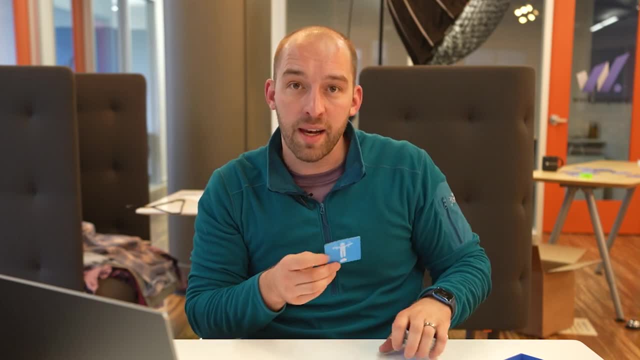 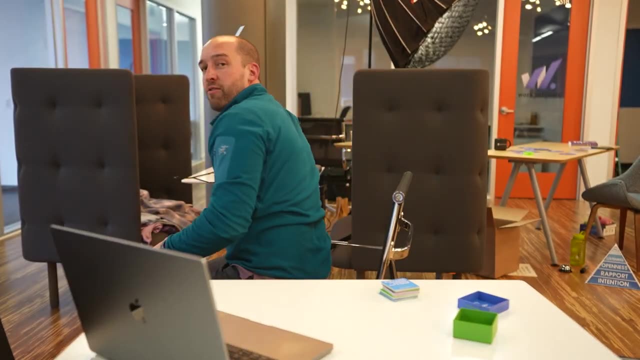 you're going to ask them the question on your card. You're going to listen to their response. After that you swap cards with that person, like Steven Swap cards, and toss your hand in the air, signaling that you're looking for a new person. So the mechanics of our, the self-facilitating 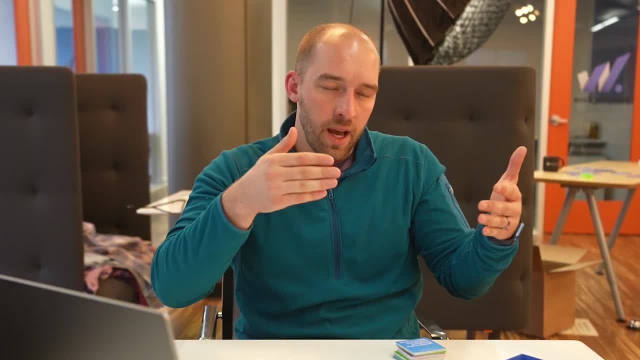 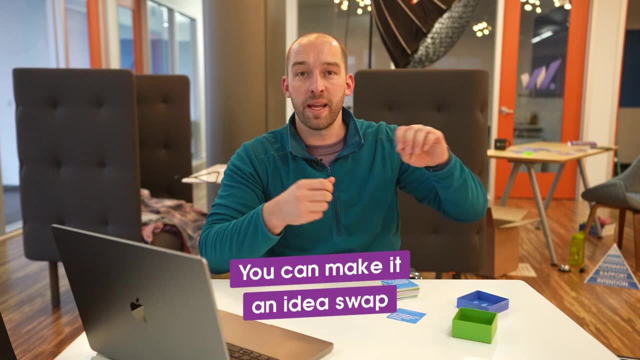 swapping. The reason it's never failed me is it allows people to be in conversation for as little or as long as they want. If you want to pivot and ruthlessly reinterpret this exercise, you could make it an idea swap. So you want to solve a problem that is currently that you're currently facing in the group Have. 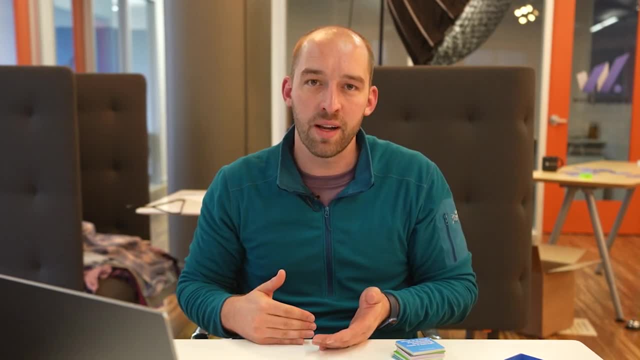 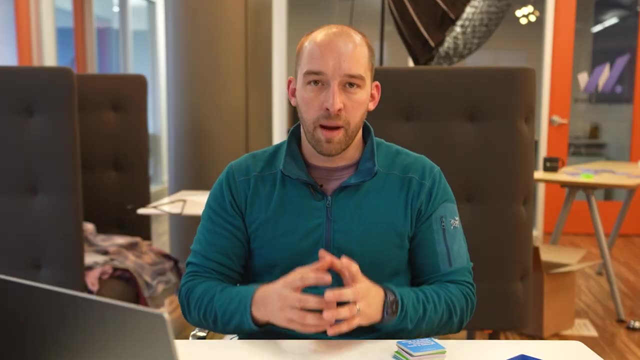 everybody write down five of their best ideas on a note card and then they stand up and they swap ideas with people and they continue doing that for about five minutes and when they come back you ask them to popcorn out and reflect what is one of the best ideas that they heard, Or if you're 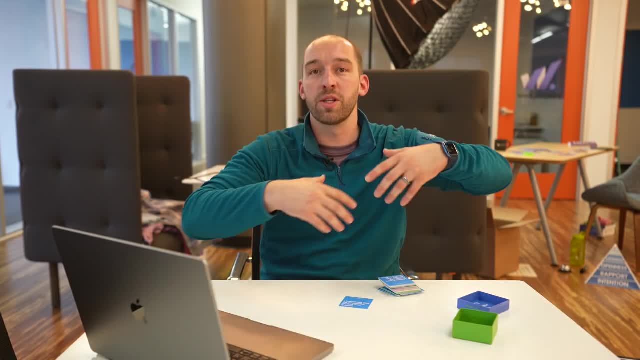 doing the question swap? what is one thing that struck you about those conversations? What is one thing that struck you about the people you're talking to? What is one thing that struck you about the people you're talking to? What is one thing that struck you about the people you're talking to? What is one thing that struck you about the people that you got to connect with? 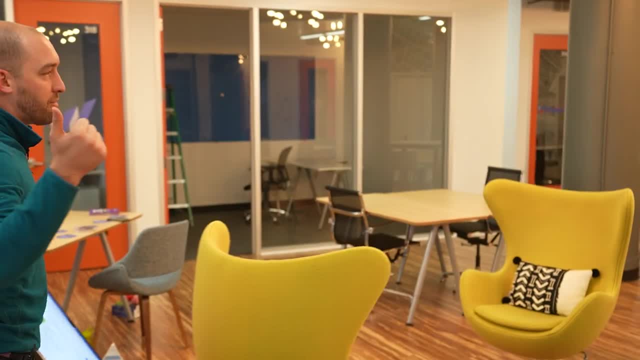 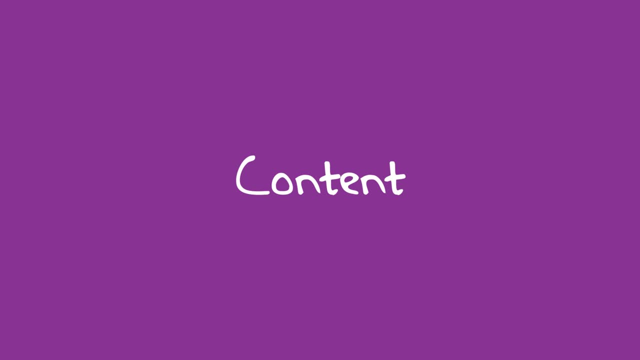 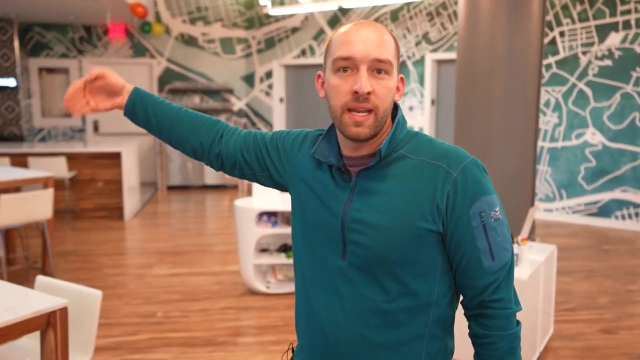 Fourth ingredient in my list of five ingredients to increase engagement is actually content, Which is a little bit weird. It's almost like can't count as an ingredient. However, I think that content for most people most of the time is 80% plus of a meeting time. right, You've got things. 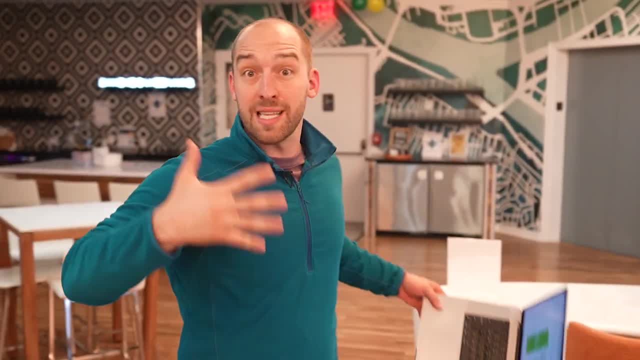 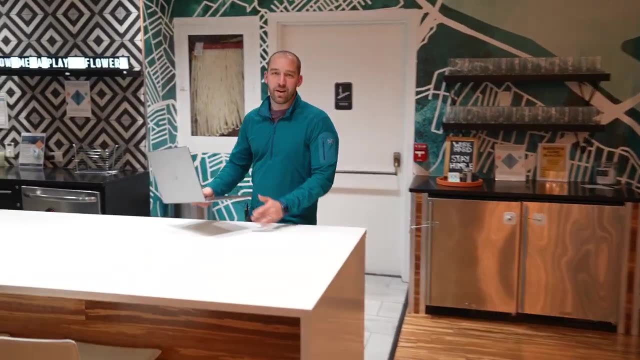 to do, decisions to make, like problems to solve, So the actual kind of slides to present, whatever else, So the Oh, look at that, Thank you lights, So the content that you're actually sharing. But ideally in my world. 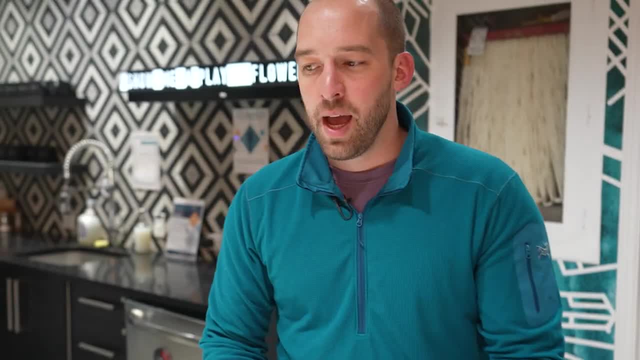 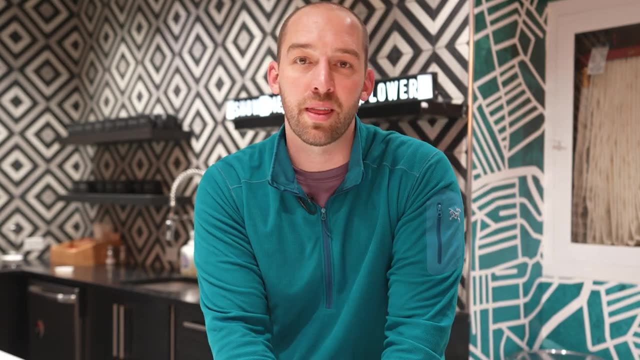 you need to design the content for contribution, And so these exercises allow you to do that. The first one: I've been saying this phrase a ton in the last couple months and it's been working with heaps of success, And it is this concept of a reaction commercial break. So 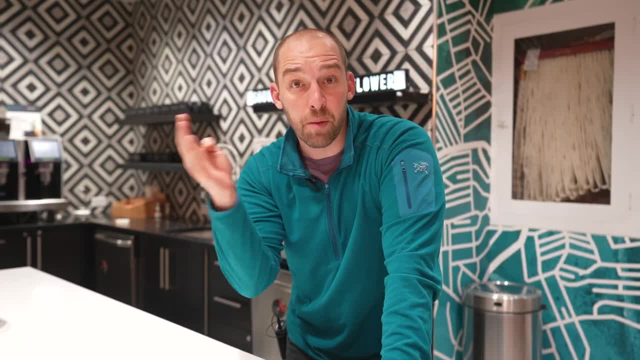 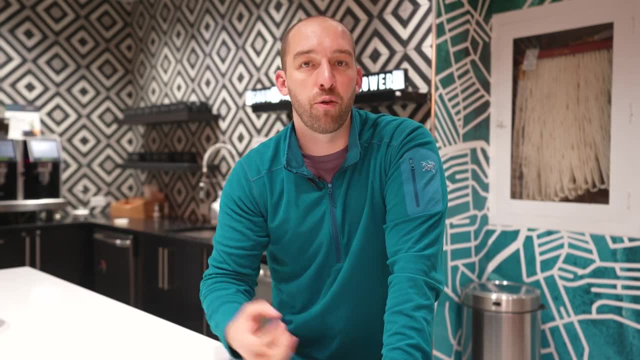 a reaction commercial break is where I've shared a piece of content with them and I get the sense that it's important for me to pause and let them digest it And also give them the platform or voice to react to it. It doesn't mean if I'm in a big group. it doesn't mean that. 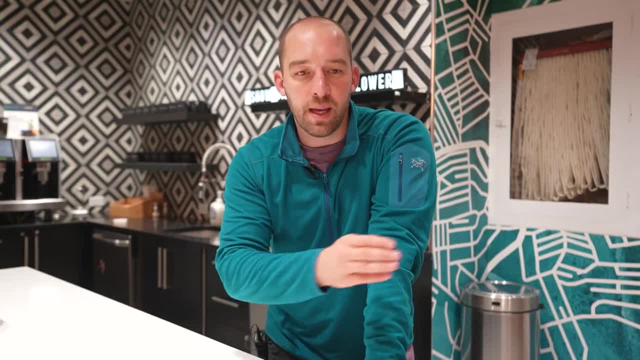 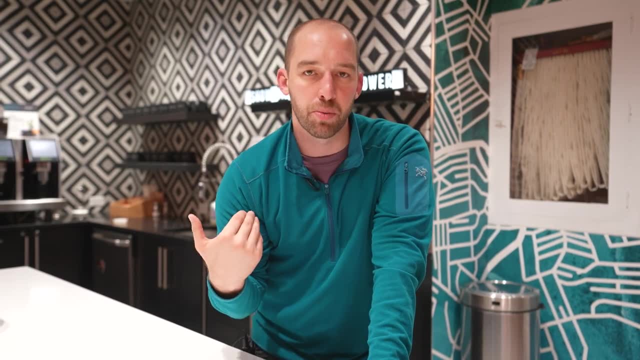 I'm letting people react to everyone. It might just be: hey, I'm going to put up the slides, share a couple ideas and then, after this, we're going to get into pairs and you just have two minutes just to have a reaction- commercial break. I just want you to share a comment, a question. 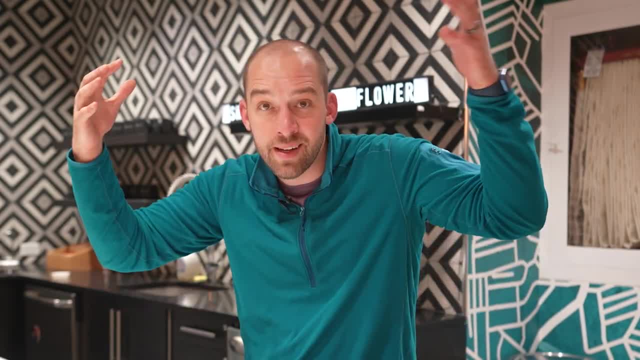 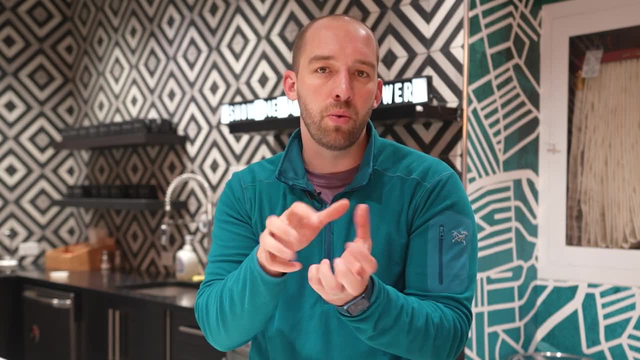 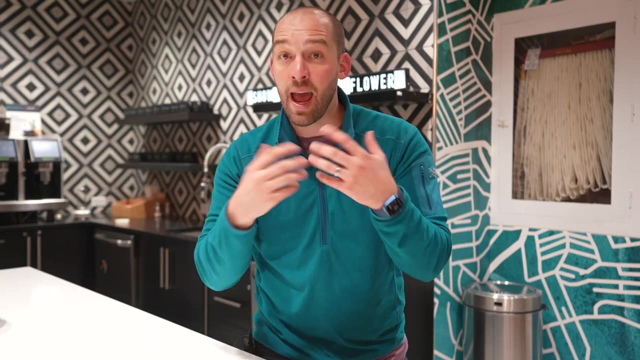 a doubt, a frustration, an excitement, an aha, Just react. So first take 10 seconds, tap into instead of silence, and tap into what is your reaction to what you just heard, and then pair up or raise your hand or get into small groups and have that reaction. It's like the purge valve on. 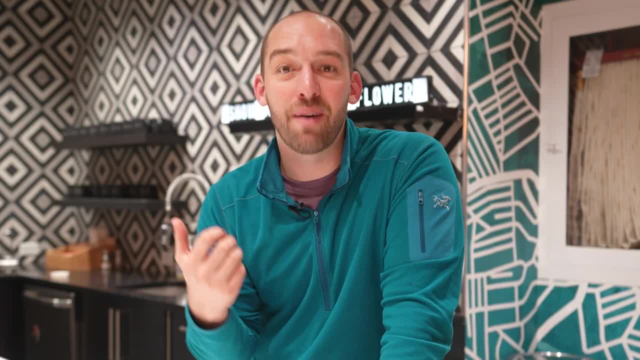 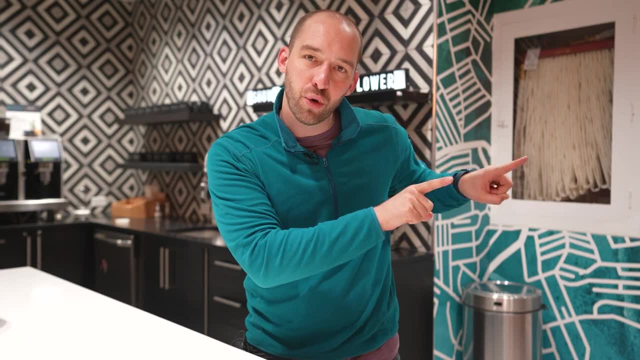 a group. If you're talking to a group of smart people for too long and they don't have a chance to react- you don't give them a reaction commercial break- it's likely that they're going to pop or explode or, more likely, slide into the role of critic. right Activity number eight: silence. 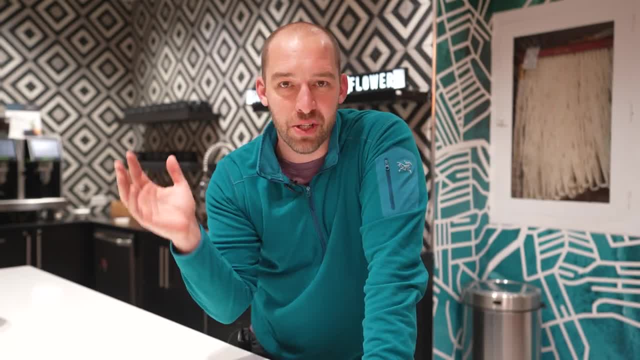 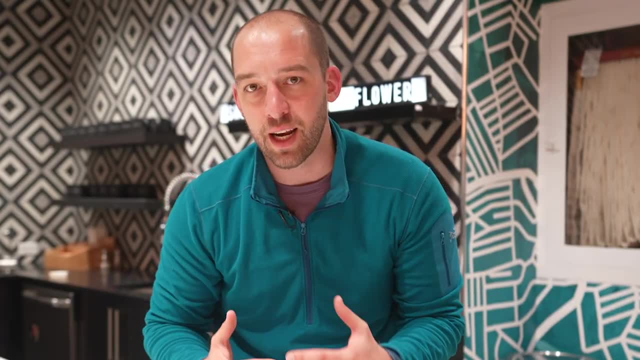 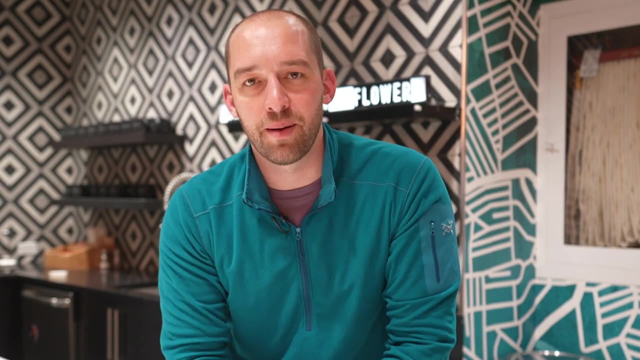 It is one of the great lost arts of conversation At Amazon. many executive meetings start with up to a half hour of silence, where all the leaders in the room are reading an executive brief or executive summary narrative of what it is they're going to talk about, be deciding on, etc. And then they start the meeting once everybody's read it. 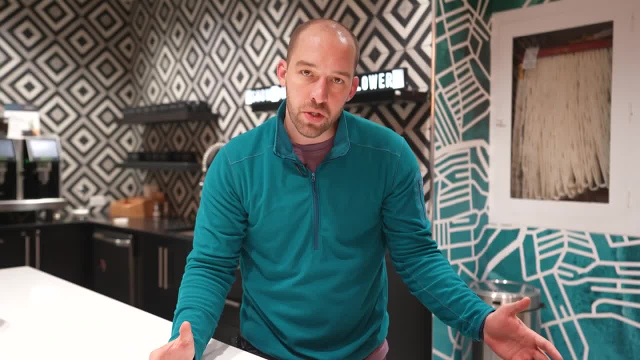 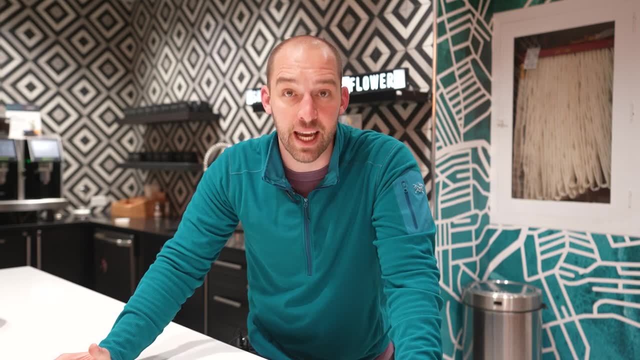 And so actually creating a period of silence. So, whether you want to brainstorm something or unpack something, creating a period of silence is one of the most powerful exercises that you can do as a group to increase engagement. It's really introvert friendly. It's also really 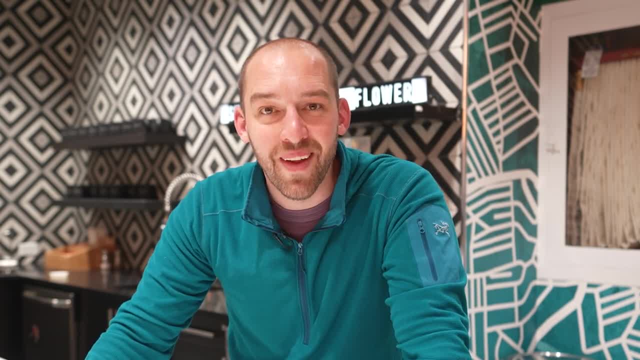 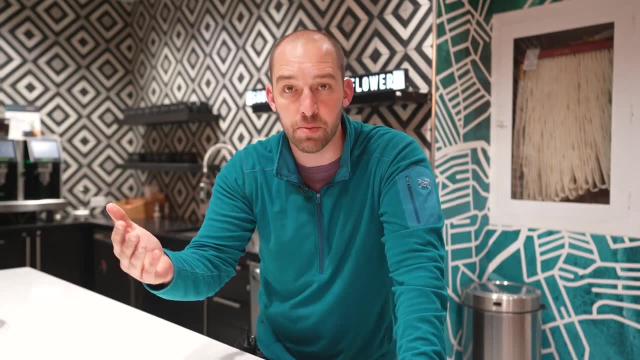 extroverted friendly. It's also really extroverted friendly. It's also really extroverted friendly Because extroverts need to shh and just listen for a minute, right. So it gives a platform to people who typically may not be the first ones to speak. It avoids groupthink. You know the idea of. 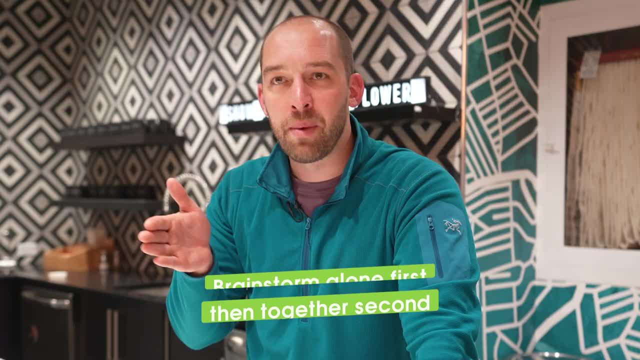 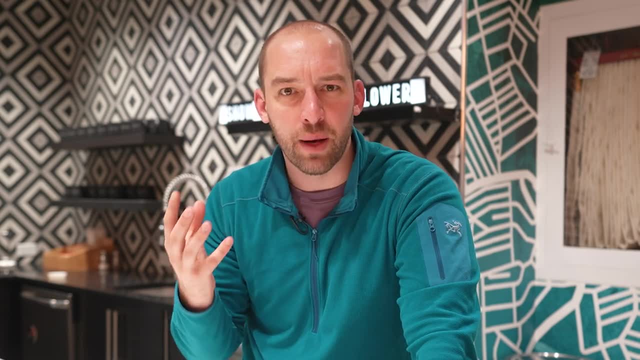 brainstorming 101 is brainstorm alone first, and together second. I'm going to take this another step forward. Brainstorm alone first, sure, tapping your own wisdom, but then, second of all Brainstorming is stupid, Like we're only tapping into what's in our brains. 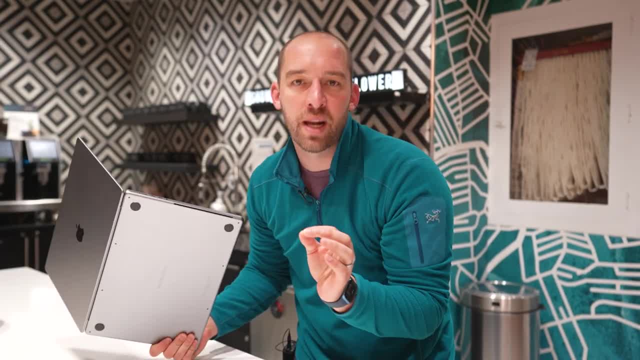 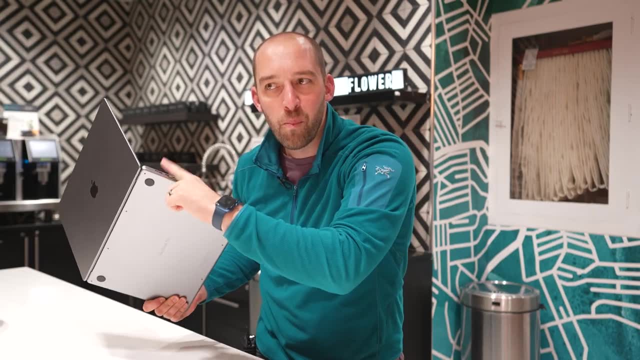 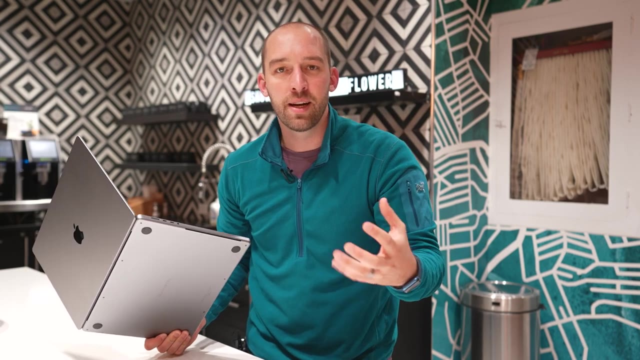 Have you met the internet? Like 0.00001% of ideas in the world exist in our brain, and so if we want to engage and create and innovate and build something really great, maybe spend five minutes of silence with everybody furiously googling the topic or purpose of the meeting to try to get some. 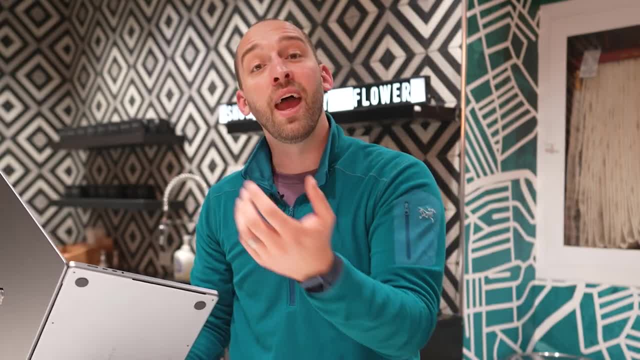 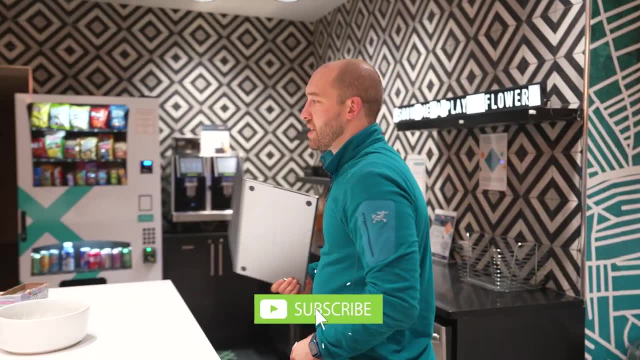 fresh new ideas injected into the mix and then meet and discuss them and share what people learned, etc. As we moved into the fifth ingredient and the two closing exercises, I just want to let you know that this video is sponsored by all the free resources in the link in the description. 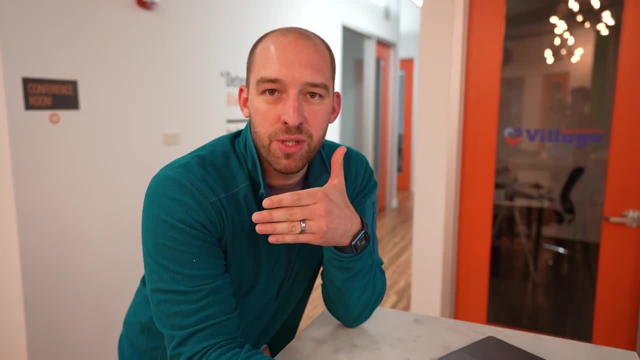 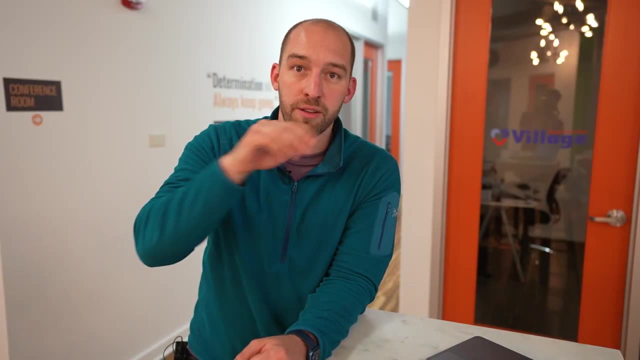 We tend to remember what happens first and last most. So if you only remember four activities from this exercise, you need to go back to the beginning and catch the first two and then you need to tune into these two, because the first and last things you do are the most likely things to 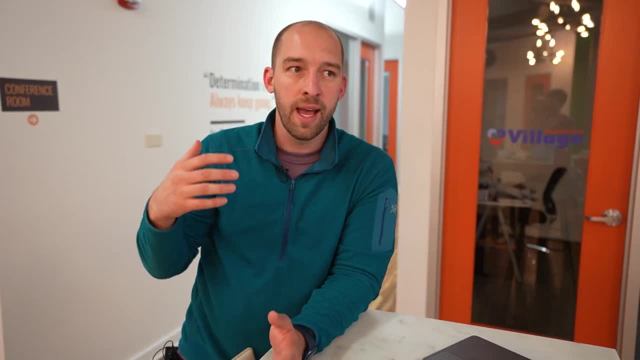 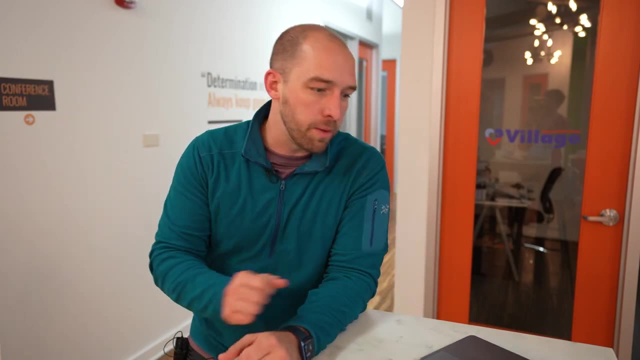 be remembered and so we've got to end. or if you want to create engagement, you need to end in a way that makes people want to come back, Whereas most gather things end in a bit of a fizzle or a rush to schedule the next time to meet One of my favorite. 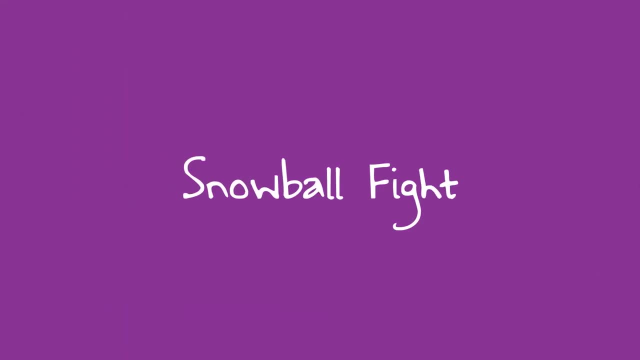 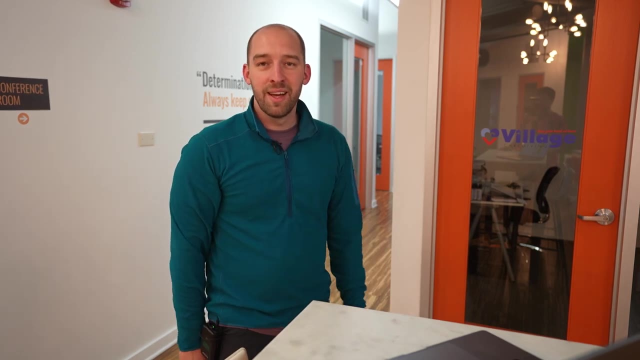 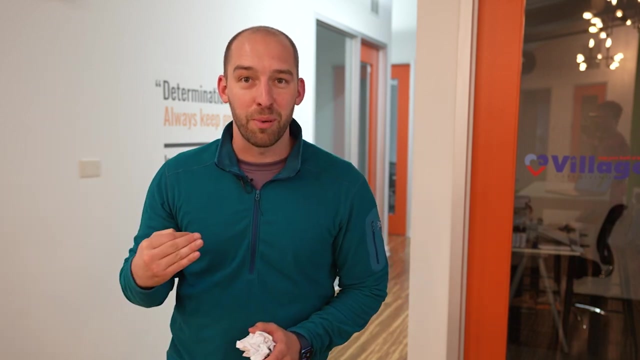 ways to close is a snowball fight. If you're watching this and you're in like a serious, technically-minded corporate context and environment which I work in often enough, right, This is still fun because tall people have the same maturity level as little people at some degree. 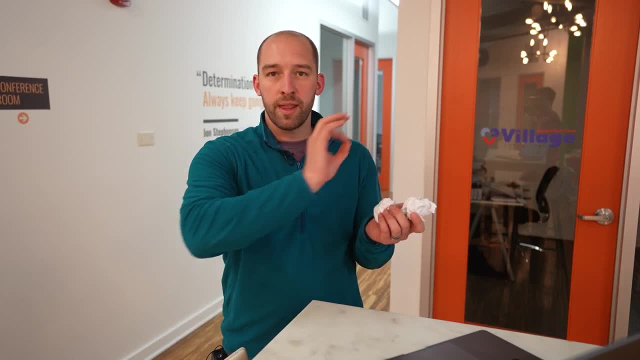 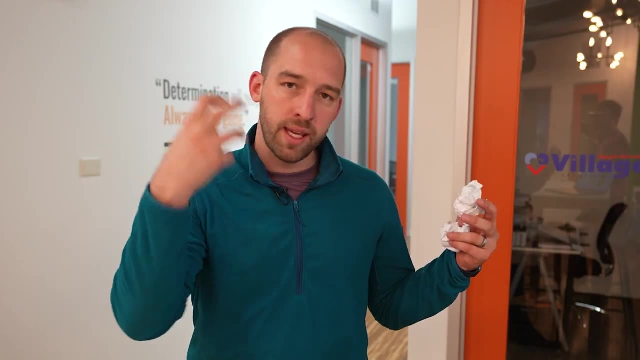 right. So really simply a snowball fight. I'm inviting someone to write their takeaway on a piece of paper, as if they're teaching it to somebody else. So write something you got out of today that was like a key point, key idea, something else. Write it on a piece of paper, crumple it up and give it to somebody else. 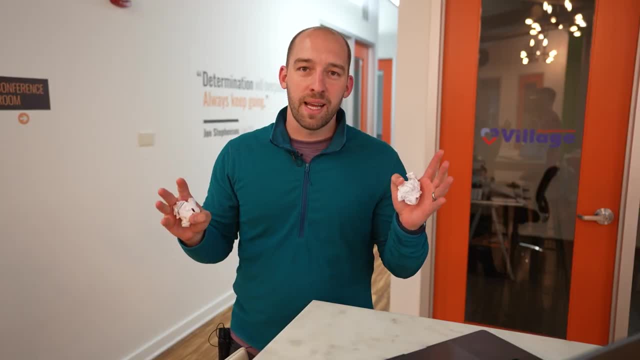 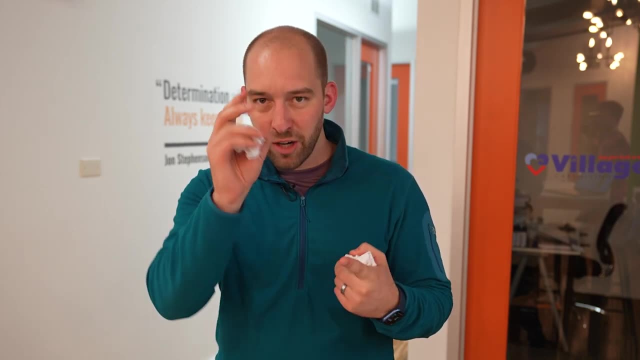 by throwing it at them and you have everybody throw it at the exact same time. and so if even if you've got seven people in the room, there is a zero percent chance that everybody in the room won't laugh or smile- Zero, right, Everybody's gonna laugh and smile When I throw this at Steven. 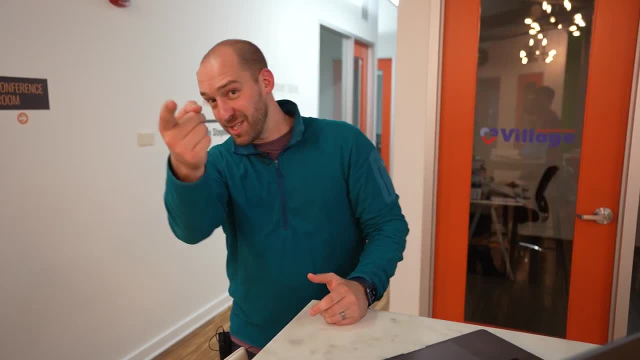 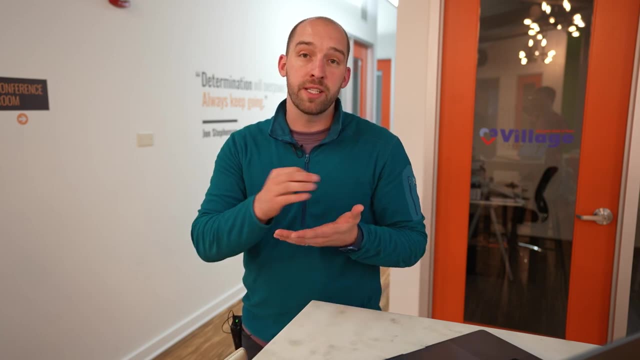 right, There's gonna be some response, some reaction. He's actually. he is smiling behind the camera. So snowball fight, So you could maybe rename it snowball gift, because the point is I wanna write something down that's gonna be as useful as possible, So I'm not writing down a like I learned a nice thing on.